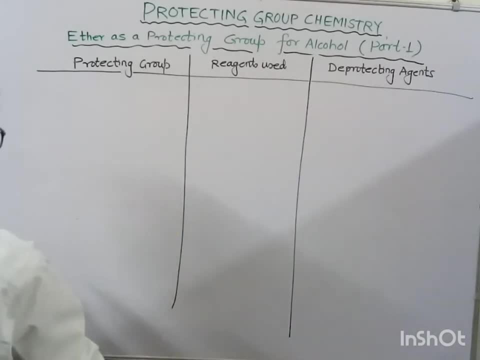 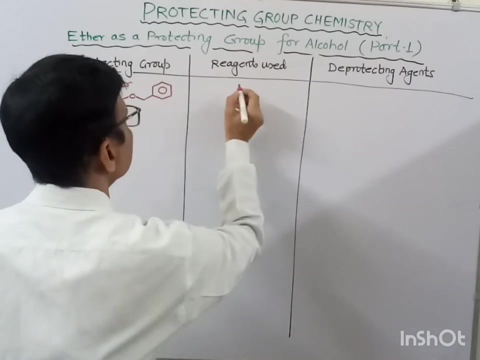 for alcohol. now, first Benji ethyl. okay, so I may write the formula. okay, so this is Benji group. okay, this is Benji ether. suppose we have we have ROH, then ROH that may react with a suitable reagent to give you the benzyl ether. so benzyl ether for the reagent, use the reagent that we use that. 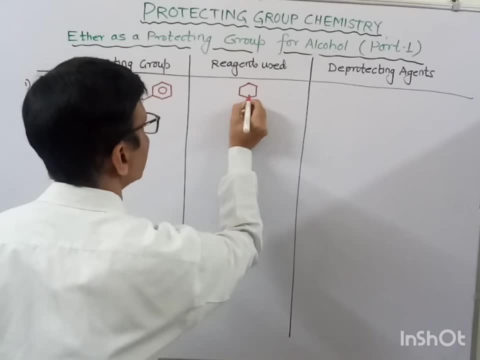 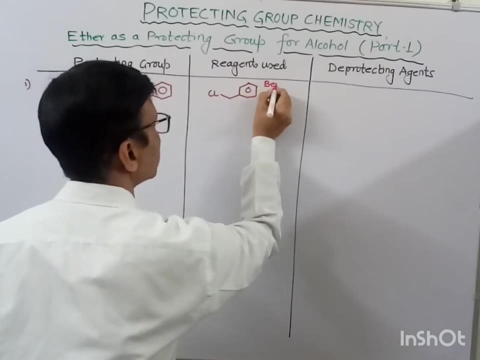 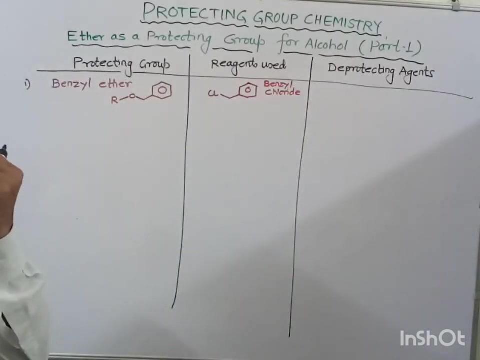 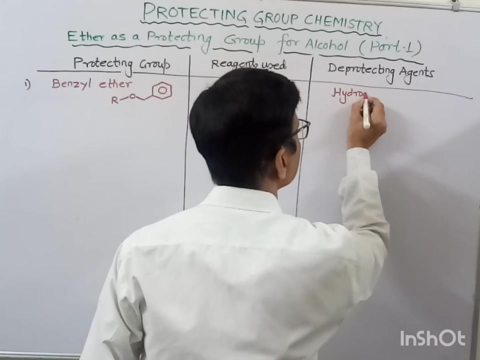 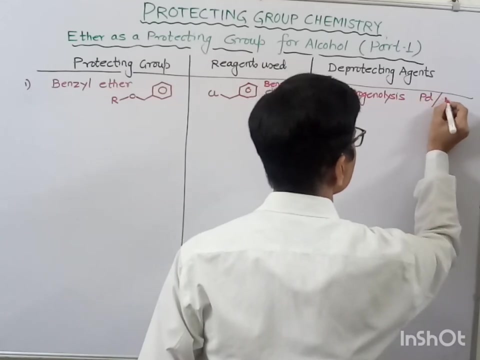 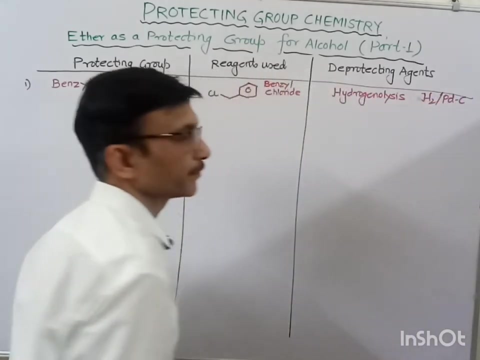 is the. we may use a benzyl chloride. we may use benzyl chloride or bromide. okay, so let me write benzyl chloride so for deprotecting this. a benzyl ether, and we do usually hydrogen analysis. hydrogen analysis, that is palladium in presence of, or hydrogen analysis, palladium charcoal. 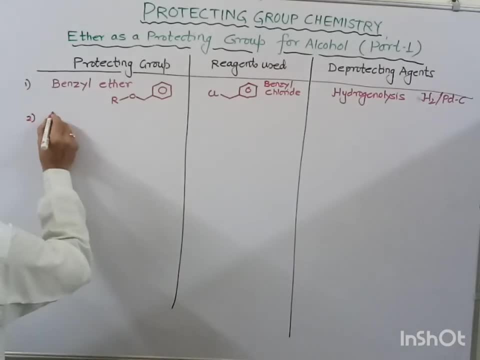 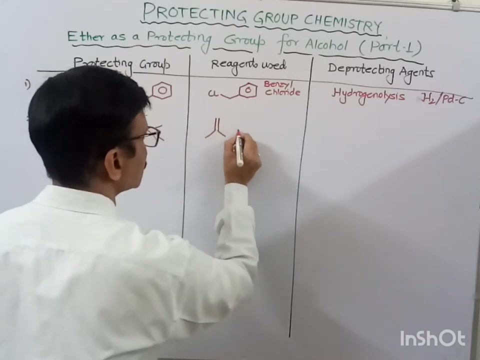 now, second one that I will tell you: tertiary butyl ether. tertiary butyl ether, okay. so the formula: okay, tertiary butyl ether, and for this we may use the isobutylene. isobutylene in presense of, we suppose I use H2SO4. 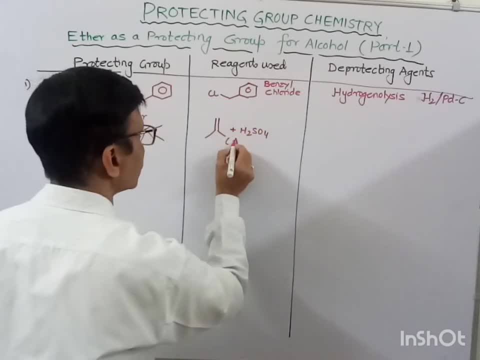 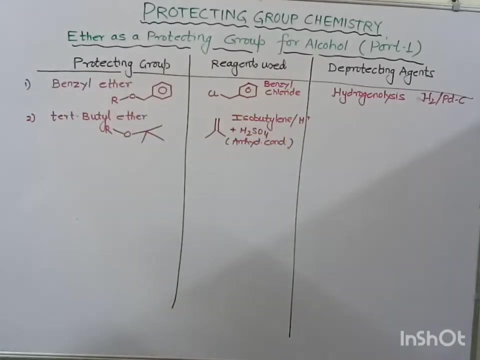 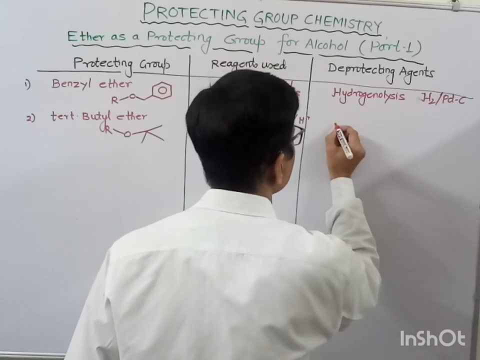 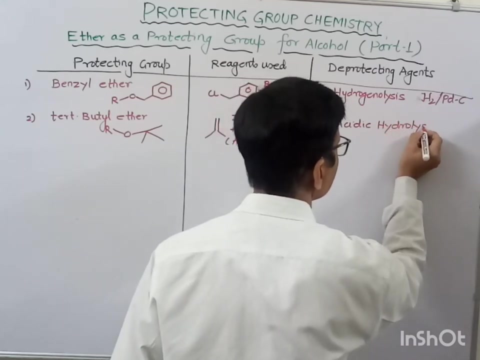 so isobutylene, and this is used under anhydrous condition. isobutylene under acidic condition- okay, so this may be deprotected. in presence of this X2SO4 ether, this acetic hydrolysis can be done to be protected. Third important one is: 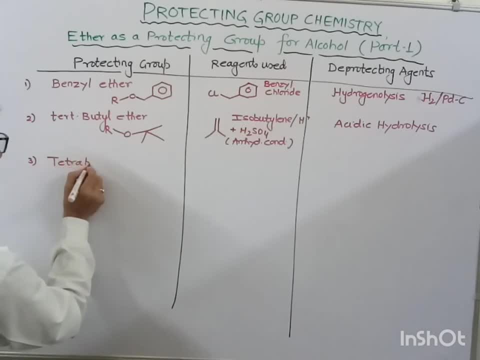 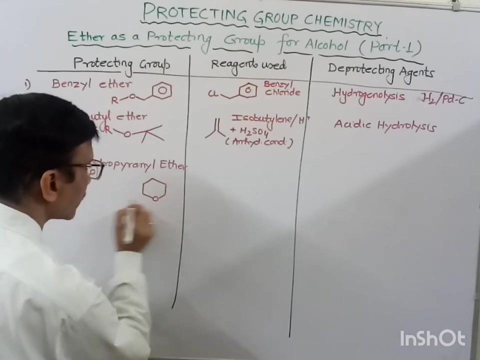 tetra hydro pyrenele ether. tetra hydro pyrenele ether. it may be written as THP, usually denoted by THP, and this is your Terry. hidro and tetra hydro pyron catches. Tetra hydro and tetra hydro pyron勝糠. 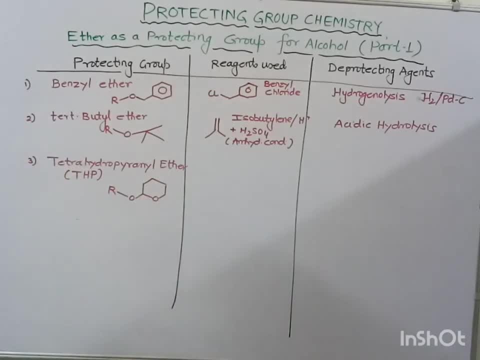 and rewrite by PH non met sometime dicen, denoting by THP. and this is your Tetra hydro and tetra hydro pyron and and this is your Tetra hydro and tetra hydro pyron and tetra hydro pyron and tetrahydropyronell ether. so if we have ROH, then it will react with the this. 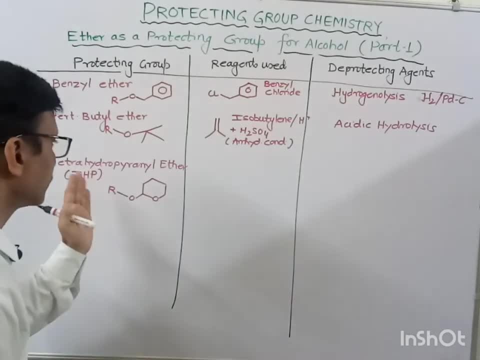 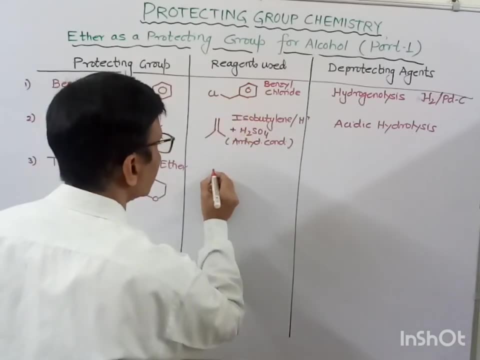 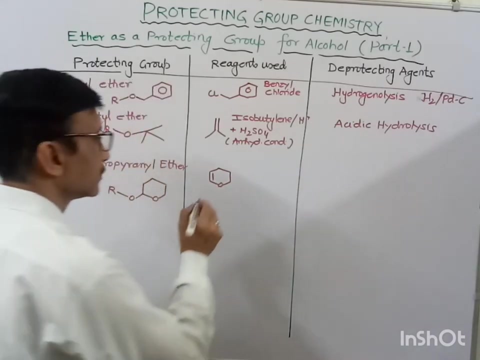 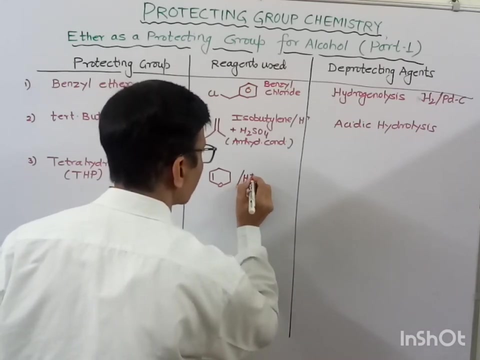 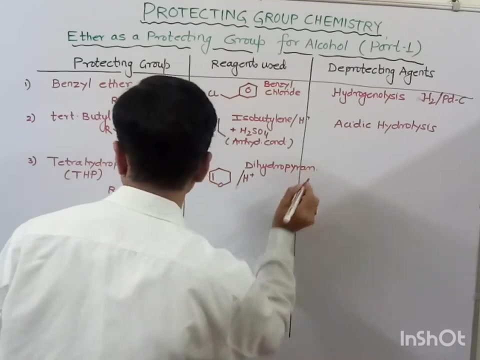 tetrahydropyronell ether. tetrahydropyronell to give you the tetrahydropyronell ether. so for this the reagent used. the agent used is we can use dihydropyronell. dihydropyronell is in presence of in acidic condition and 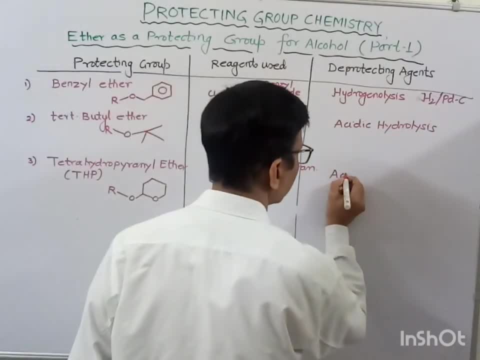 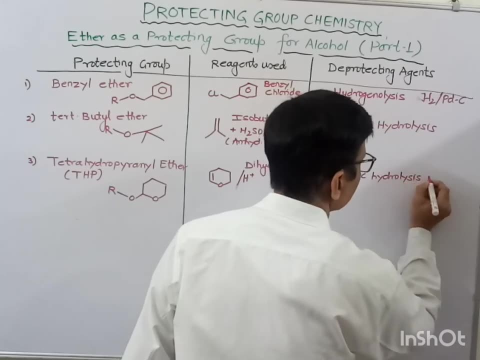 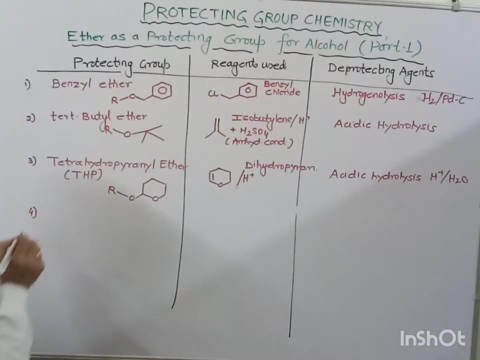 to be protected. we may do the acidic hydrolysis. again, we may do the acidic hydrolysis. okay now, fourth one, fourth important one, is trialkyl silyl ether. trialkyl silyl ether- okay so trialkyl silyl ether- we may represent it by this- is R1, R2, R3, R4. 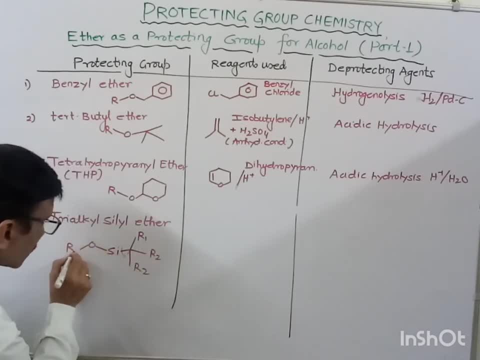 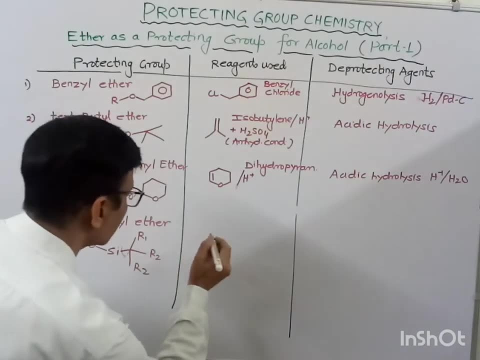 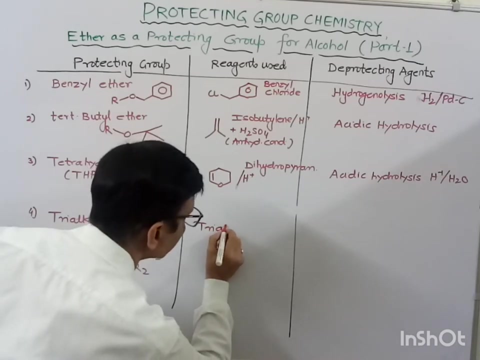 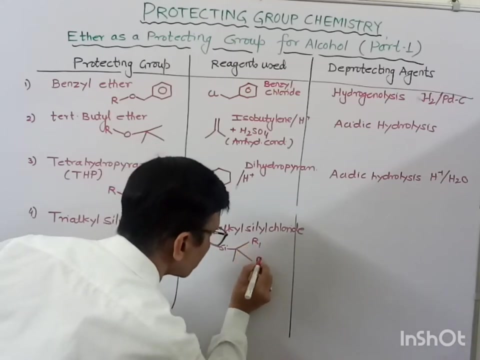 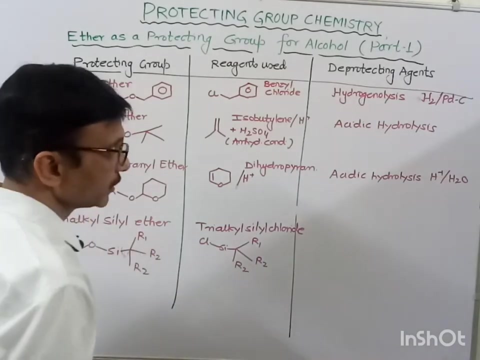 ok, so R1, R2, R3- it may be different alkyl group may be present over here, and so for this we can use a trialkylsilyl chloride as a reagent- trialkylsilyl chloride- and for this deprotecting agent we use a particular deprotecting agent, and it is 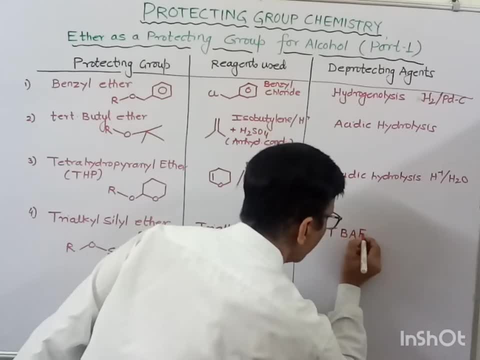 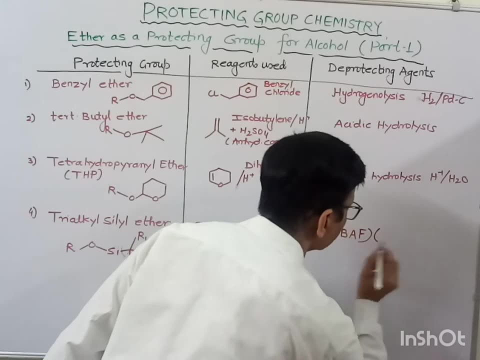 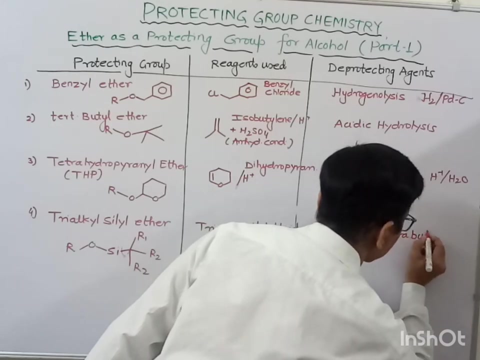 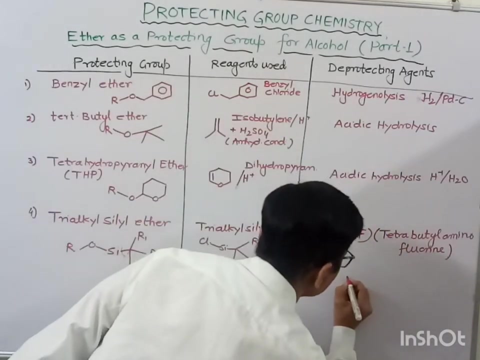 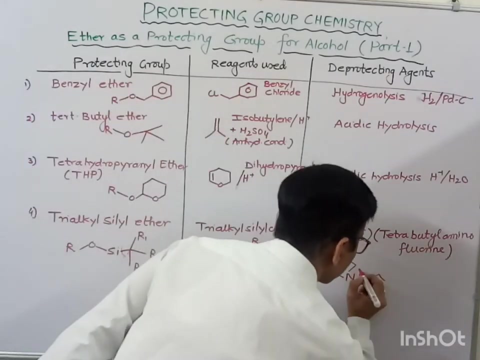 named as TBEF. okay, so TBEF is a protecting agent, so we may write it that is tetra butyl trialkylsilyl chloride aminofluoride. so the structure, if we may write the structure. so this is tetrahydromine and this positive charge over here and this is 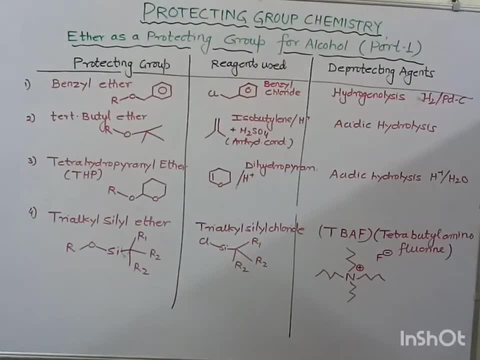 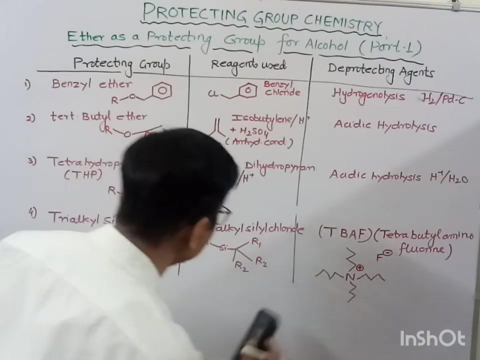 fluoride, and okay, so we may have a different type software. trialkylsilyl ether. so if we see different trialkylsilyl ether, and let me give you the different formulas, trialkylsilyl ether, so it may be, it may be, suppose this is one of the. 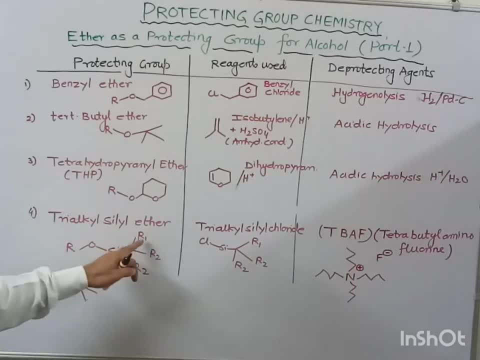 if we may write methyl group, if all this, really this, is a methyl group. so if we and this R1, R2, R3 are the methyl, then this is trimethylsilyl ether. You may write it: trimethylsilyl ether. 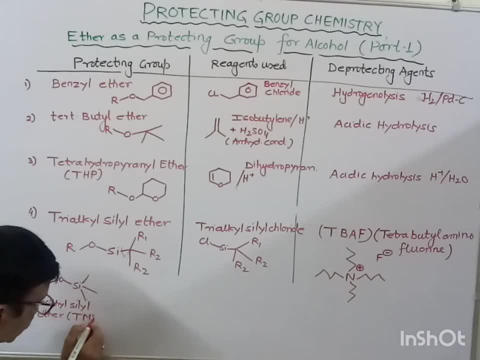 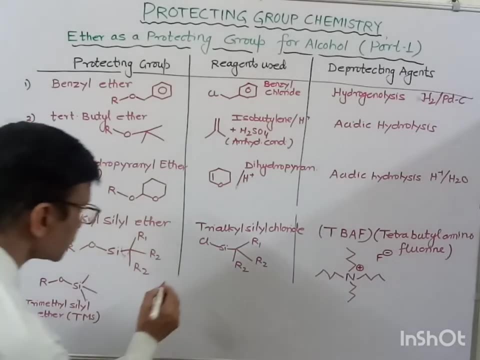 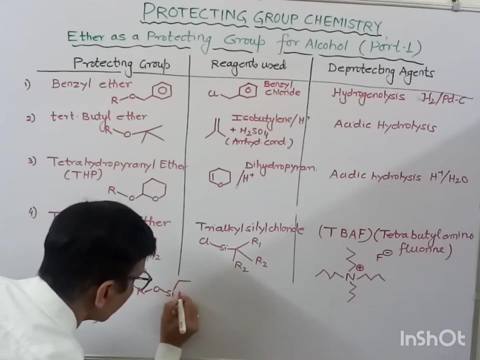 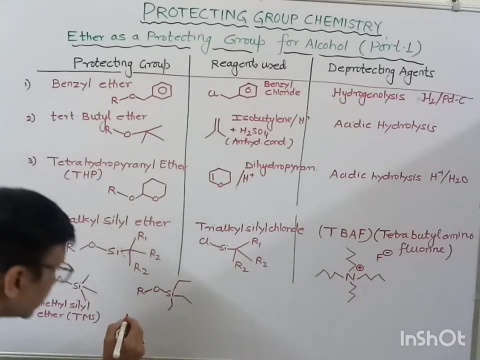 Okay, it is TMS, trimethylsilyl ether. In the same way, if ethyl group is present, suppose if ethyl group is present, then we may write it. we may write it. trimethylsilyl ether. trimethylsilyl ether. 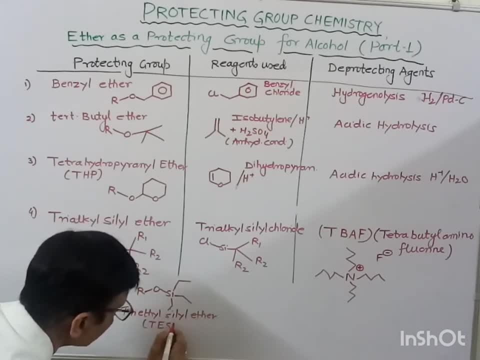 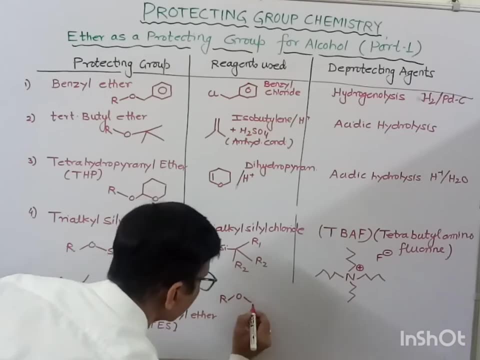 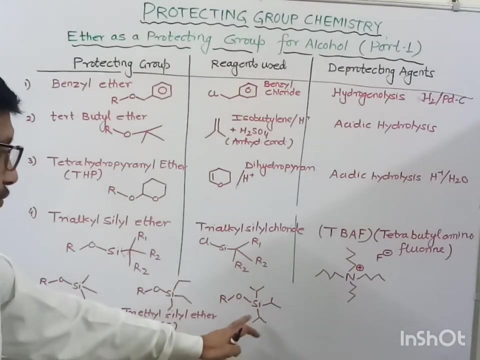 Okay, trimethylsilyl ether TES. In the same way, suppose if we have, we may have isopropyl group, We may have isopropyl group. So if isopropyl group is present, then it is triisopropylsilyl ether. 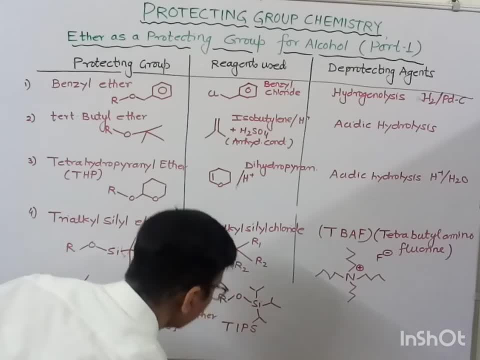 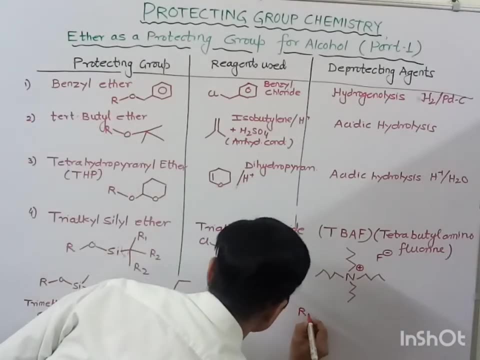 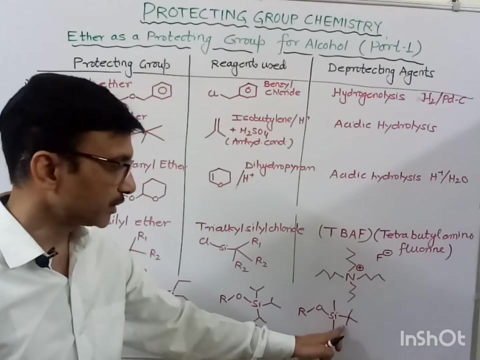 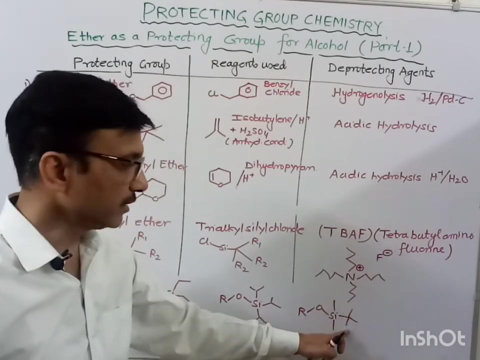 Okay, triisopropylsilyl ether TIPS, TMS, TES TIPS, And then another one we may have. two methyl groups are present and one tertiary butyl group is present, So it is tertiary butyl, dimethylsilyl ether. 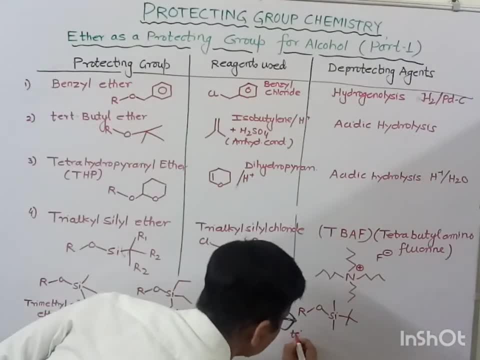 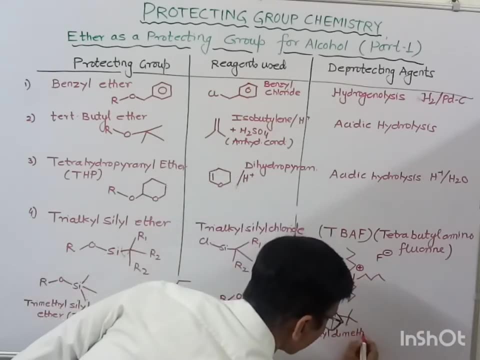 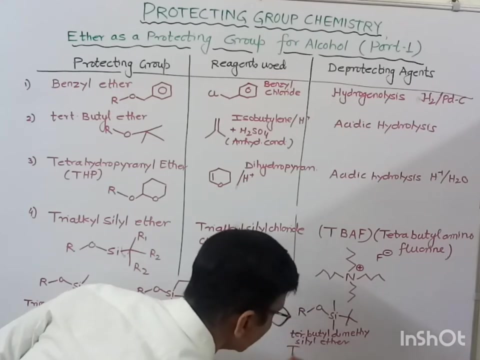 Okay, it is tertiary butyl. Okay, it is tertiary butyl dimethylsilyl ether. So we may write it as tertiary butyl dimethylsilyl ether. Okay, it is triisopropylsilyl ether. 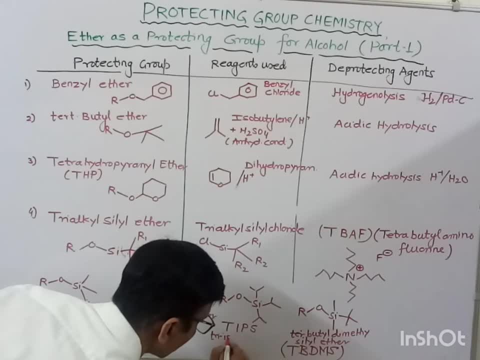 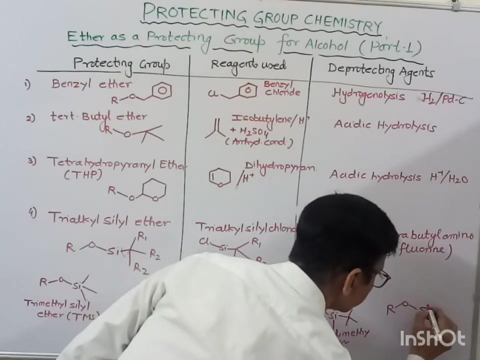 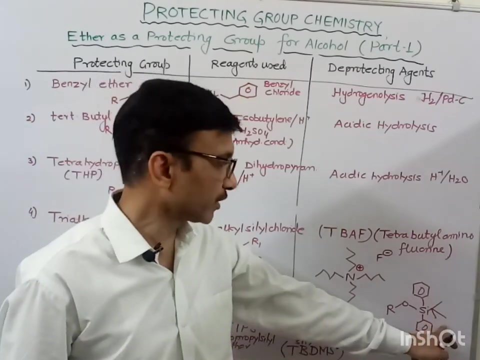 Okay, this is triisopropyl, And next one is tertiary butyl. Okay, so here one group is tertiary butyl and the two groups are the phenyl, So it may be written as tertiary butyl. Okay, so here one group is tertiary butyl and the two groups are the phenyl. 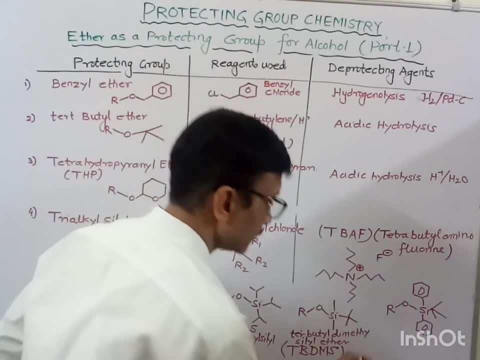 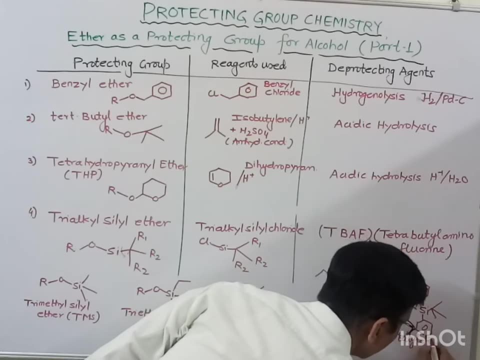 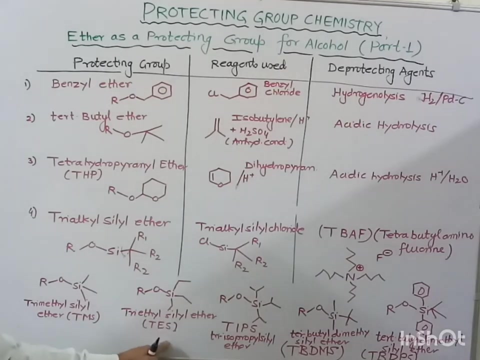 butyl diphenyl selide ether. it may be written as tertiary butyl dimethyl selile ether and it is T: tertiary butyl TB diphenyl, TPS, TB, DPS. okay, so TMS, TES, TIPS, TB DMS, TB DPS. so these are the 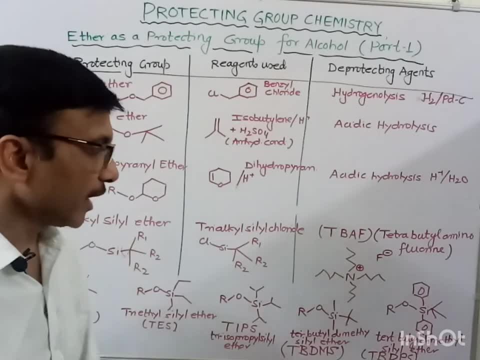 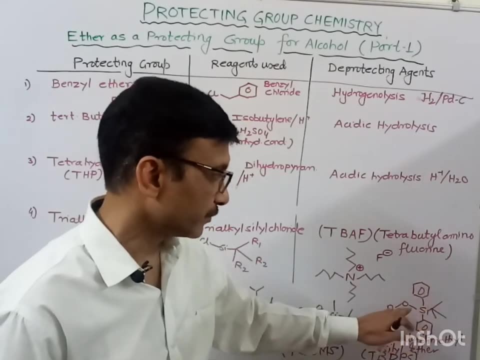 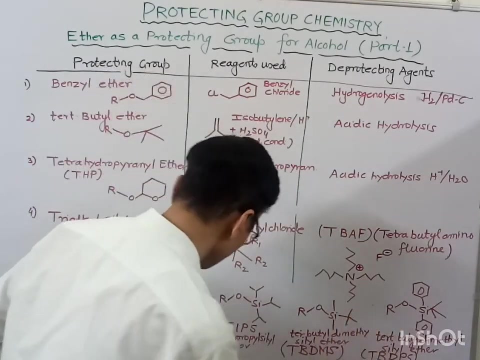 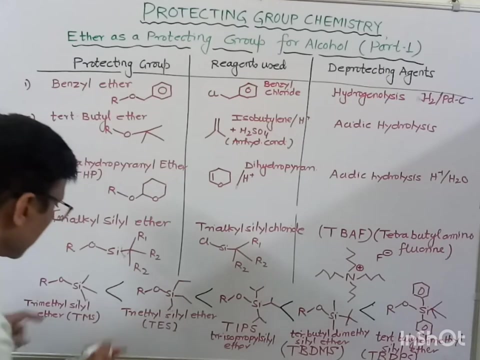 different forms of a trialkyl selide ether and if we see the stability, then it is. it has the bulkiest drop over the silicon, so that's why this is most stable. this is most stable. if we see the stability, then this is most stable and this is having the least bulkier group. 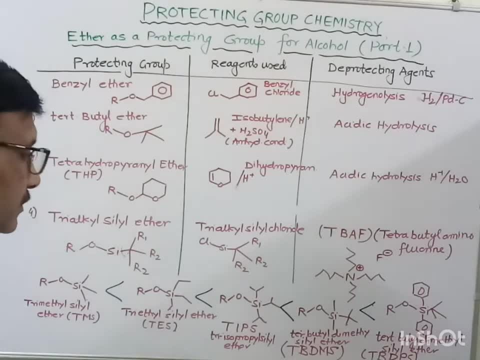 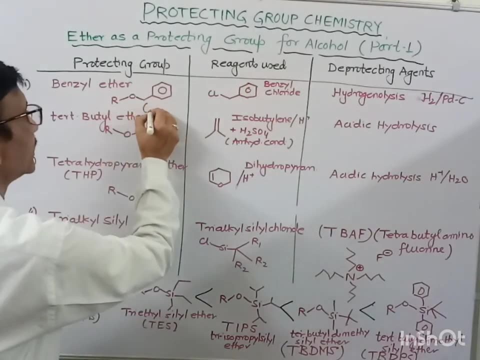 that's why this is the least. so this is a stability order. so we have benzyl ether, so benzyl ether, you may write it. sometimes we can write it as a R- R-O-B-N. This is BN, means benzyl ether, R-O-B-N, Or sometimes we may write it as a R-O-B-H. 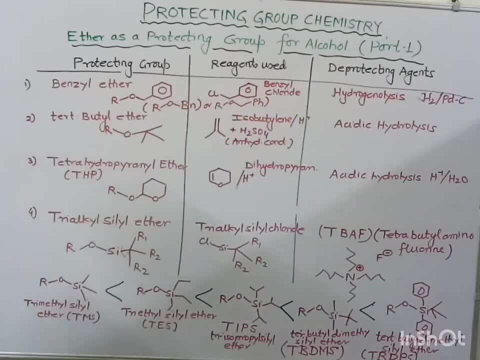 This is benzyl ether. This may or may not. Anyway, we can write it So: benzyl ether, tertiary butyl ether, tetrahydropyronell ether, trialkyl silyl ether, and these are the various. 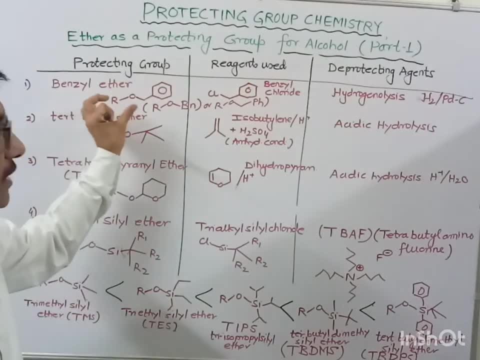 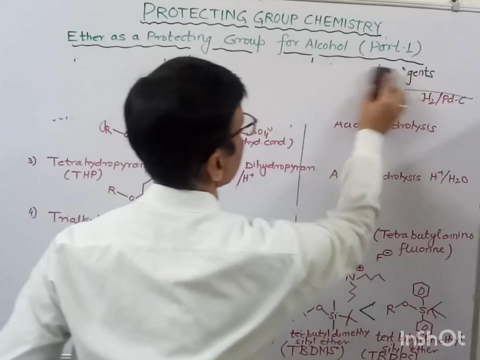 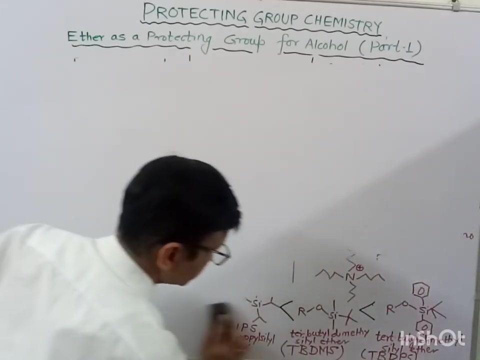 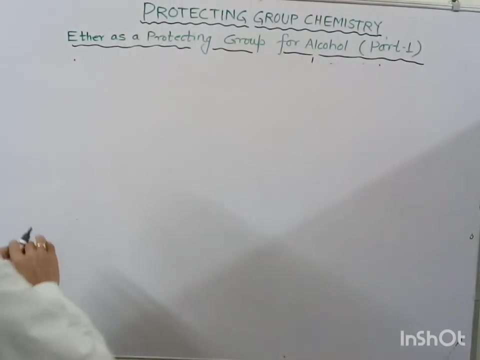 reagents used to protect this alcohol, and this is the various tea protecting agent for this. Now let us see this one by one. Let us see the benzyl ether. First, I will discuss the benzyl ether. Let us see the benzyl ether. 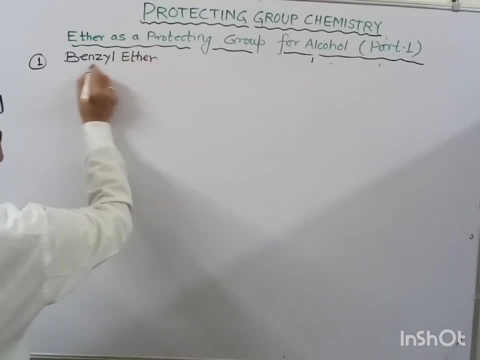 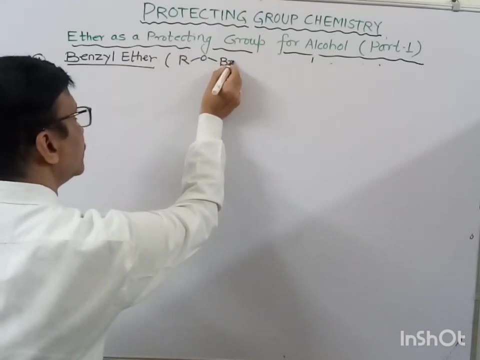 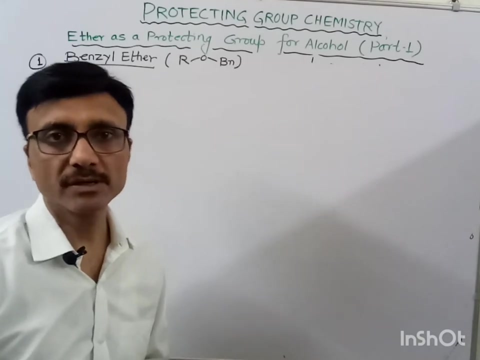 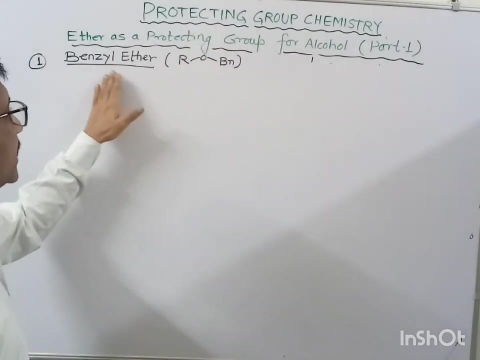 Benzyl ether. Okay, So we may write it as a R-O-B-N And tea protecting agent used is the hydrogen palladium charcoal, And the hydrogen illicit of this bond will be R-O-B-N, R-O-B-N, So this is benzyl ether and the agent used to get this benzyl ether, that will be the benzyl chloride. 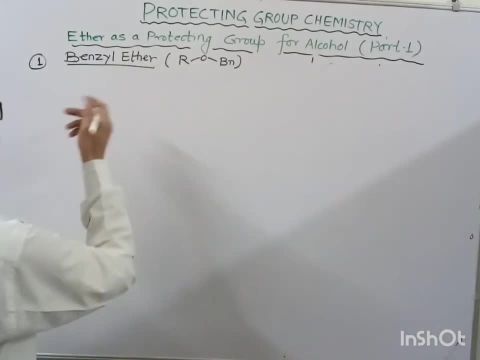 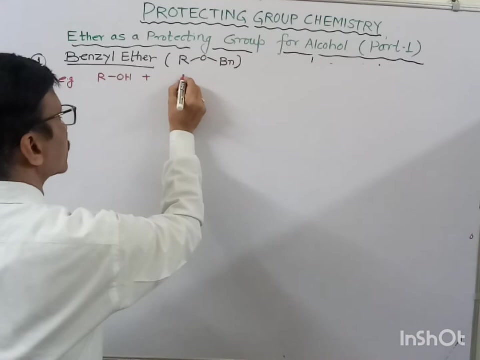 benzyl chloride may be used. So let us see one of the example. So let us see the example. So suppose, if we have in a general way, suppose this is R-O-H, So this in presence of benzyl chloride. 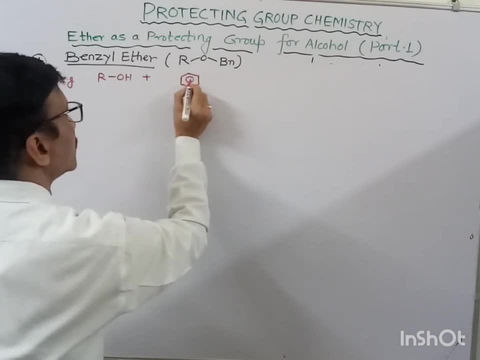 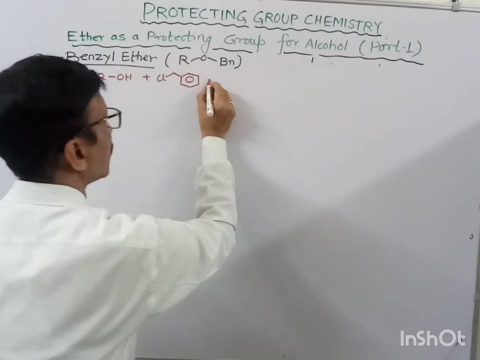 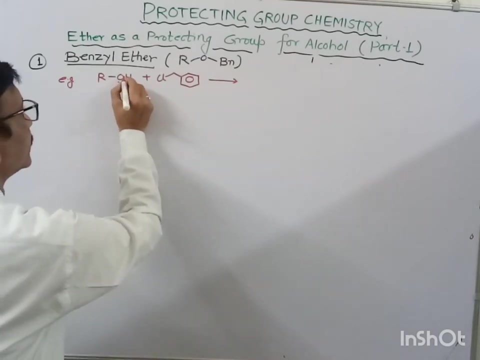 in presence of benzyl chloride, So this will form a ether. So this may occur in presence of either sodium hydride- if we write- sodium hydride may be used to to extract this acidic hydrogen from here. And what we may get, We may get. 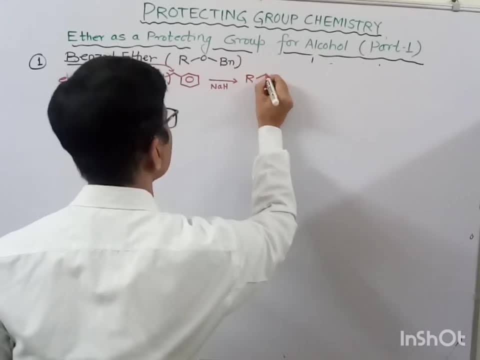 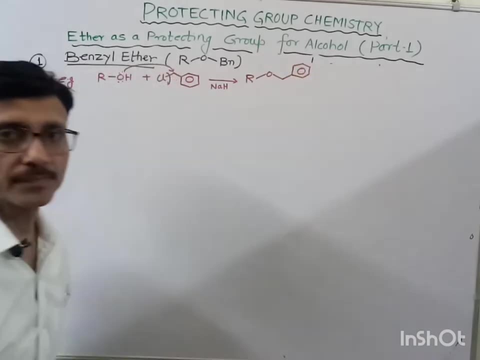 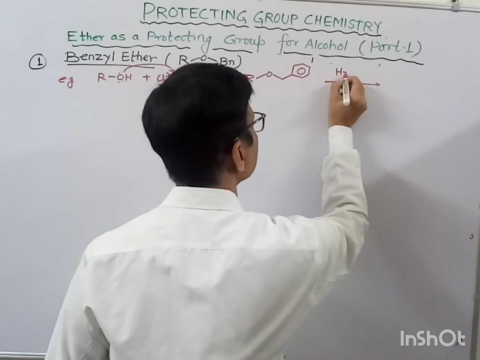 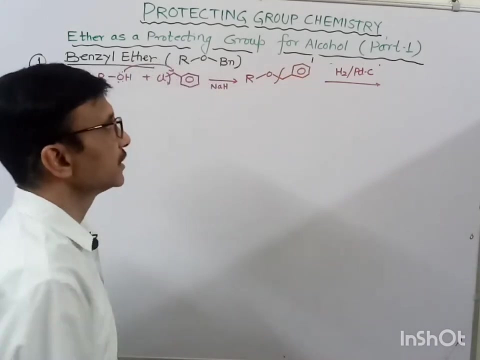 So this one Like this, And so this is the protection and further the deprotection can be done. So for deprotection, hydrogen, palladium, charcoal, hydrogen, illicit of this bond will takes place. So H, one of the H will come over here and the H here. 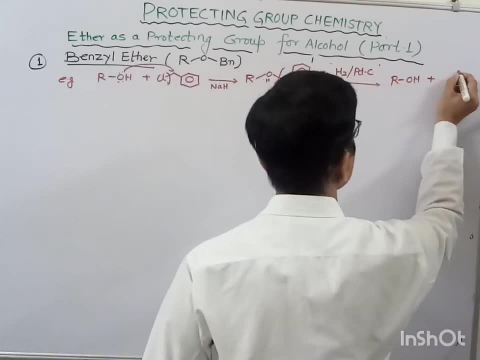 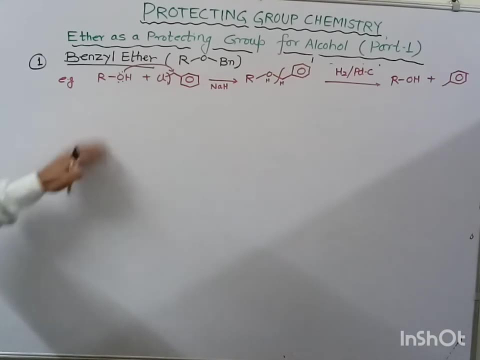 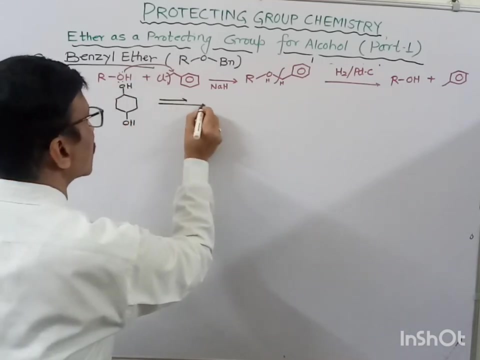 So R-O-B-N, R-O-H, we will get again R-O-H and we have the okay Now. so now let us see one of the example. So if I write one of the example, if we have a suppose this conversion, if we have suppose this is a conversion and we have to convert it into 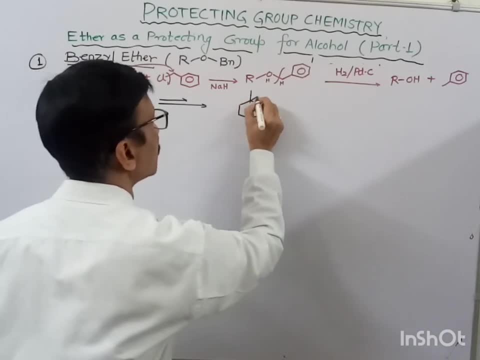 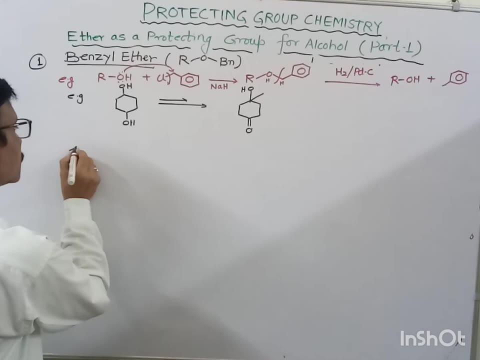 into into into into an LUP. First let us see the conversion. Okay, So we have two OH Group, So first of all I will protect one of the OH Group. So, with the help of this Benzyl chloride, so we may use, suppose, sodium hydride to extract. 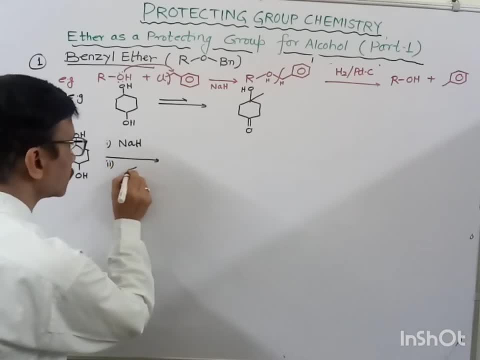 this hydrogen, acidic hydrogen- then we may use the benzyl chloride. okay, we may use the benzyl chloride Now, after this extraction, after this extraction. okay, so this will extract this hydrogen hydride ion, will extract this hydrogen and here, this having a negative charge. 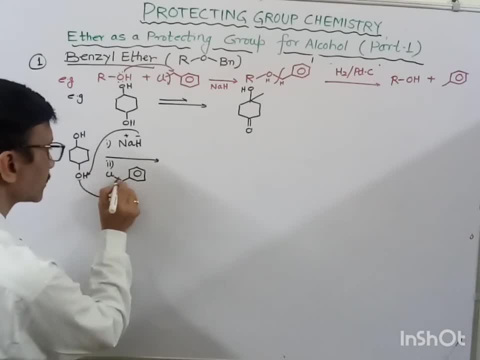 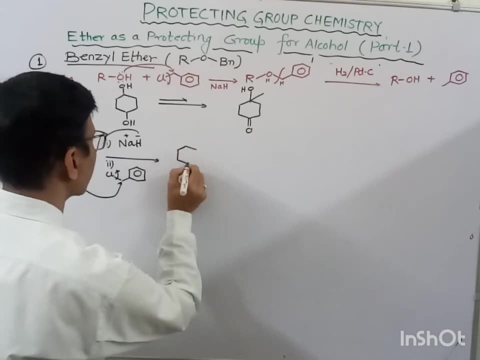 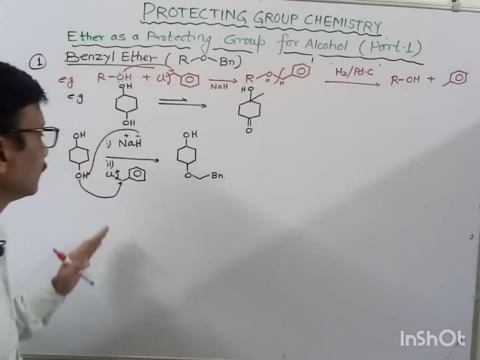 this having the negative charge, this will attack over here and this chlorine will get out. So what we will get, We will get here this OH and this OBN. I may write it BN, benzyl, benzyl Now. so here we will use only one equivalent of this. 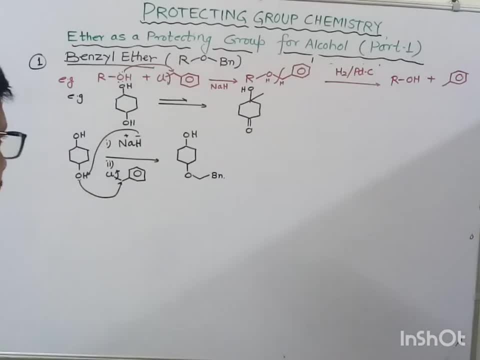 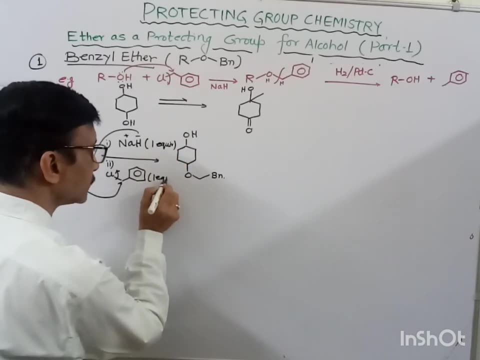 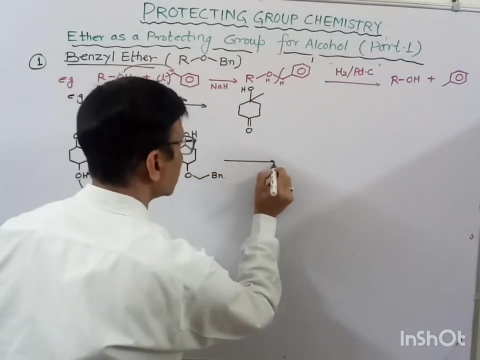 so that, so that only one OH is protected. So let's see, let me write it one equivalent of this, And here also one equivalent of this, okay, So that only one OH get protected. And now this OH, this can be oxidized. So if we oxidize it, we may oxidize it with. 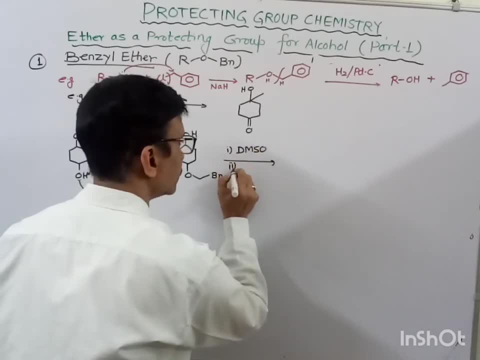 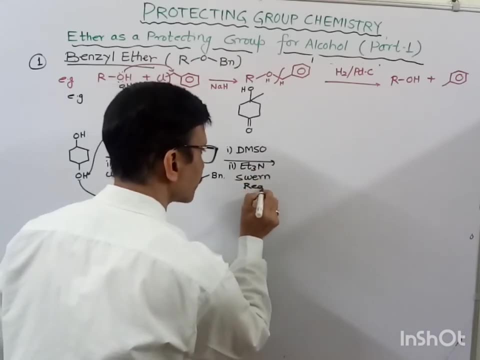 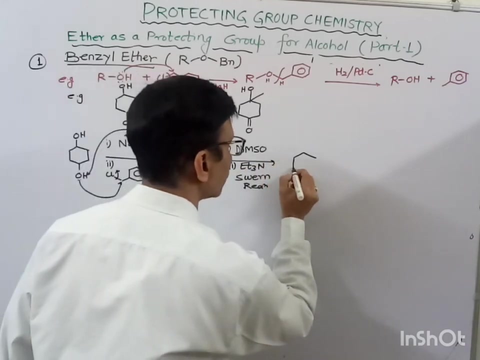 the help of this DMSO and trithylamine, and this is the Avioswans reaction, So this will get oxidized. This is a secondary alcohol. So, as this is a secondary alcohol, that could be converted into ketones and we 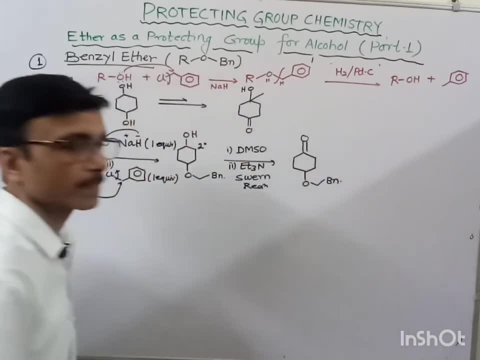 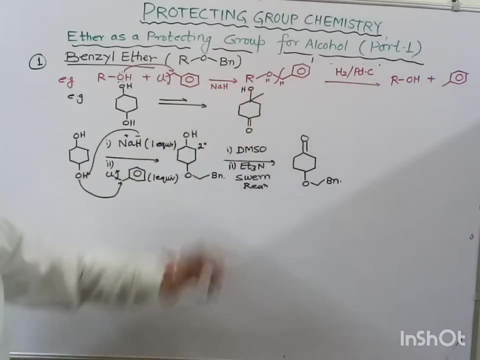 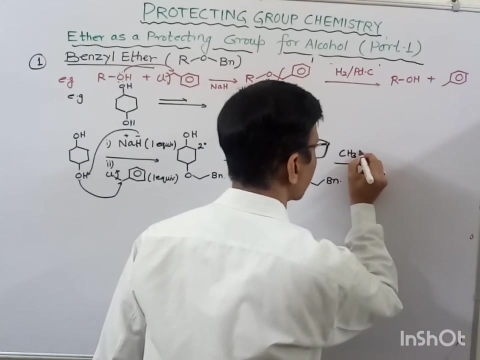 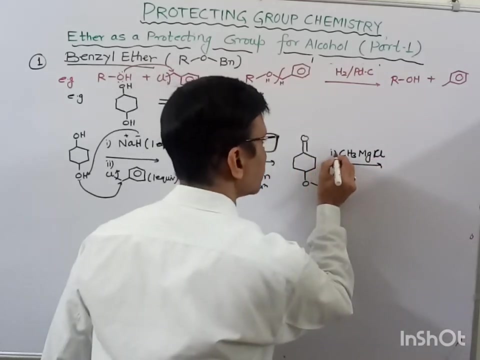 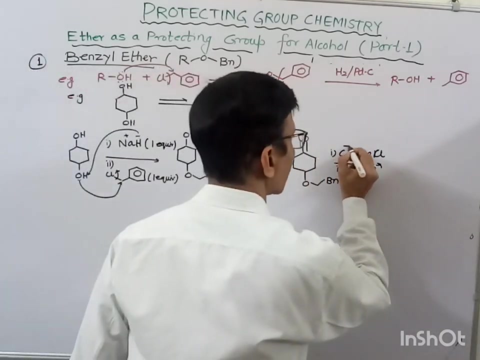 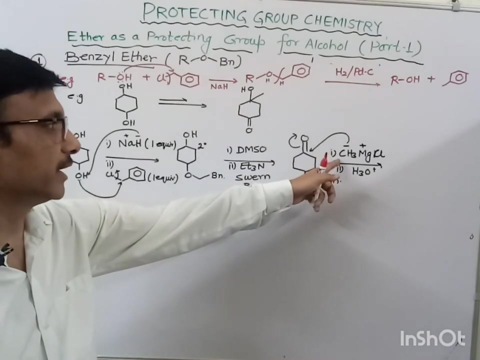 may have here benzyl group, Okay now. so here we have to get this OH and this methyl group, and this may be done after the nucleophilic addition of this is the NR reagent. So we may do this, Followed by this hydrolysis. So what we may get. So minus plus. so here CS3 minus it will. 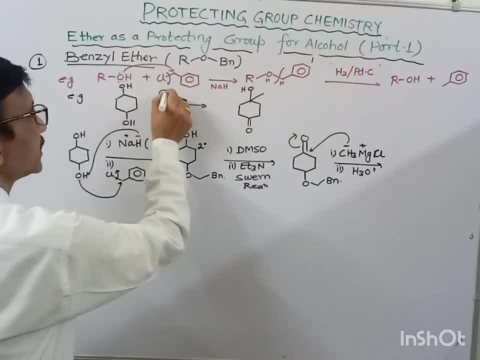 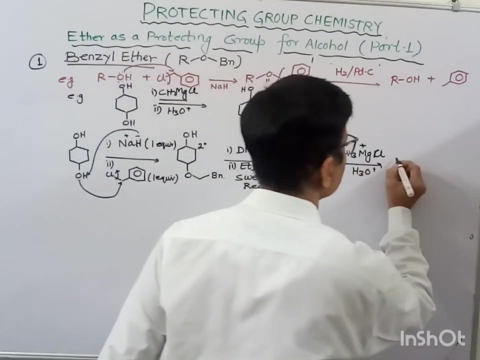 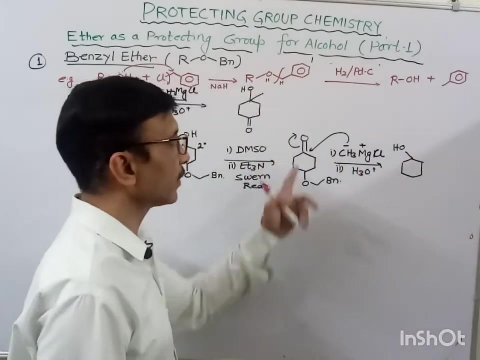 act as a nucleophile and it will add over here. Okay. So suppose if we have a CS3MgR, so we may write here, we may use this reagent and this one hydrolysis, So that means we. So what we get here, this would be after hydrolysis. this would be O minus. that would 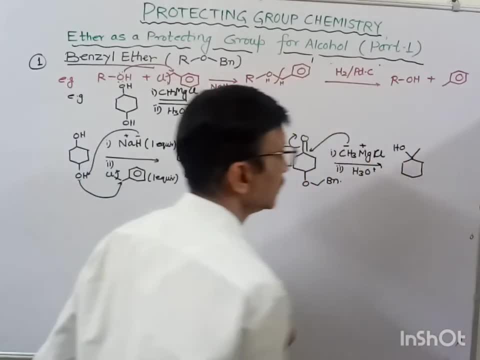 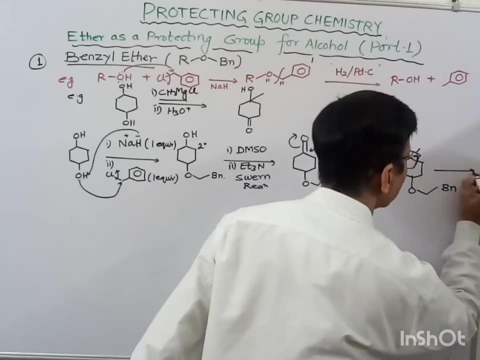 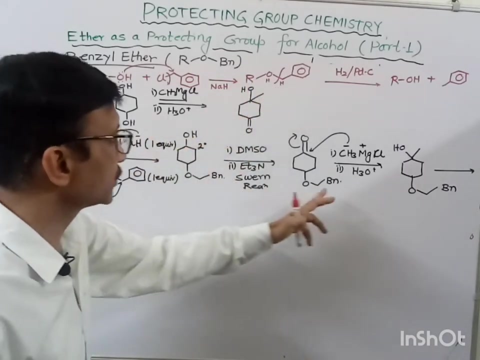 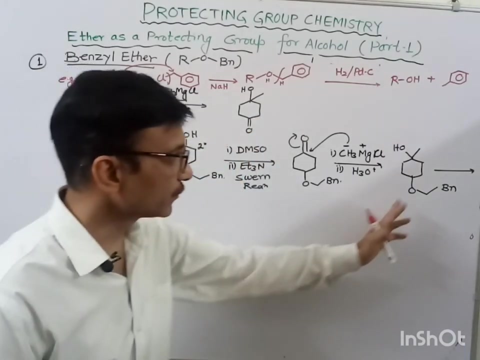 be converted into OH, and here we have one of the methyl group and now this is the benzyl ether. Now what we can do here now? so we have got this portion, now this OH. now we have to get this ketone over here, so this should also be oxidized. So for that, first of all, we will 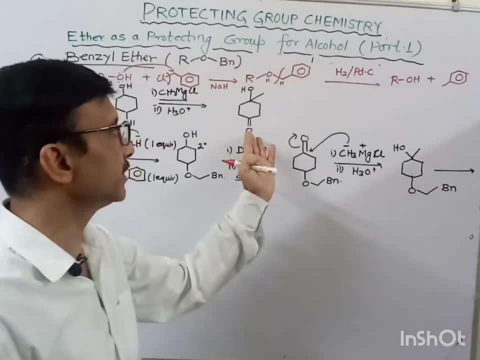 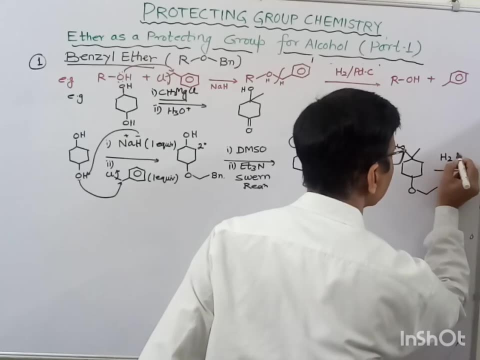 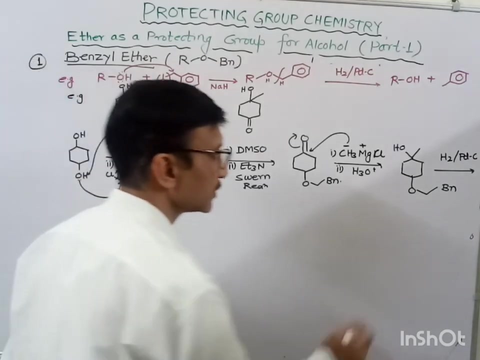 deprotect it and after deprotecting we will oxidize to get the ketone over here. So now let's deprotect it. so deprotection with the help of dehydrogenolysis network, so the hydrogen analysis that will be here and this would 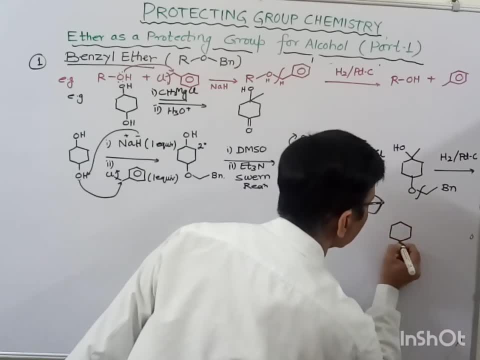 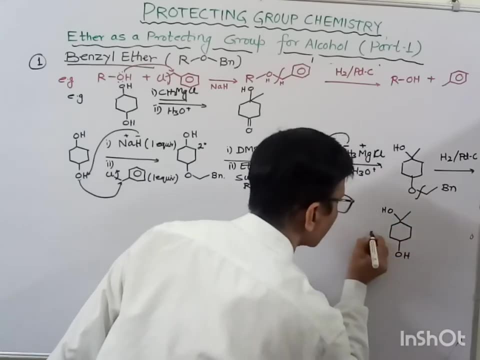 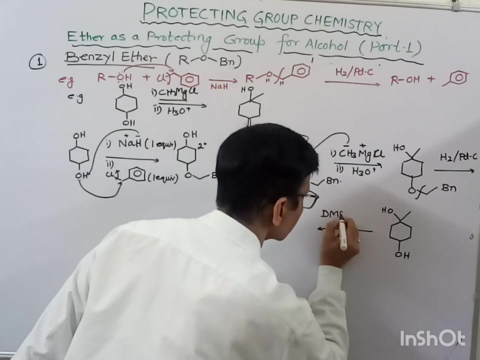 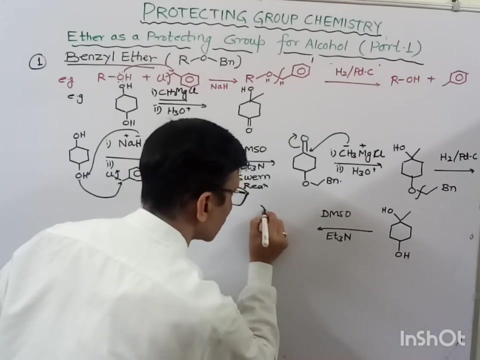 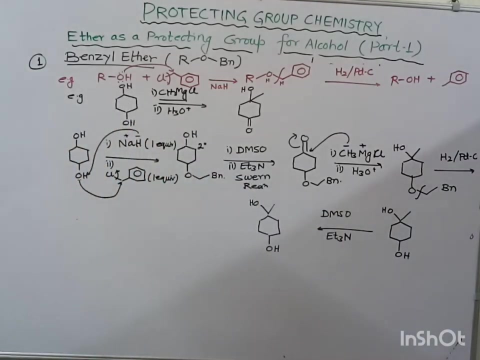 get broken and we will get here and here. OH, Now again that can be oxidized using this swans reagent, swans reaction, DMSO and this trithylamine and we will get our DMSO product. now we are getting the design okay, so like this. so this is one of the 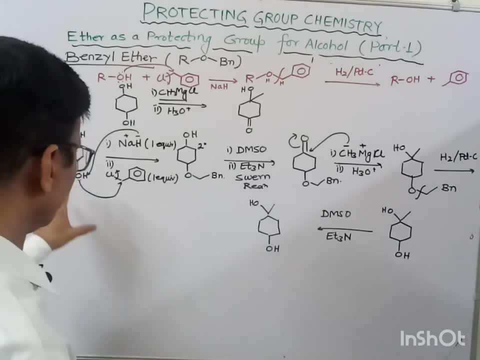 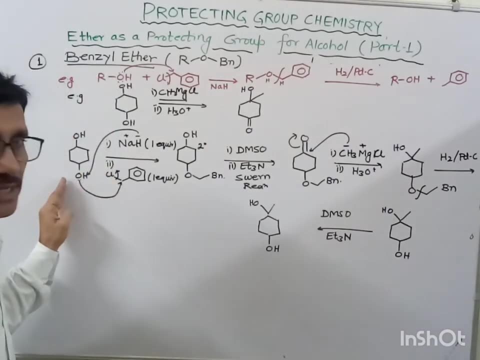 example. now suppose here this protection is necessary, first one of the wedge groups that should be protected. so suppose if we do the oxidation then both groups will undergo oxidation, both group will undergo the both group, both watch will convert into this keto group. and if we reacted with it, not reagent, then here 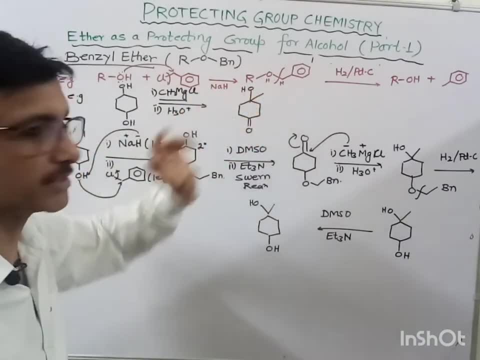 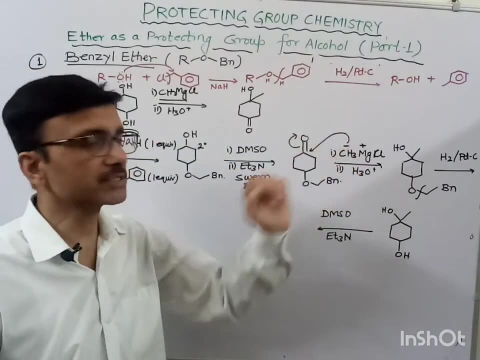 at both. this position we have is watch and with hell you practice position. so that's why, first of all, we should protect one of the wedge group and then the new click addition reaction of this will not region can be done, and further deprotecting it and after deep protection again, 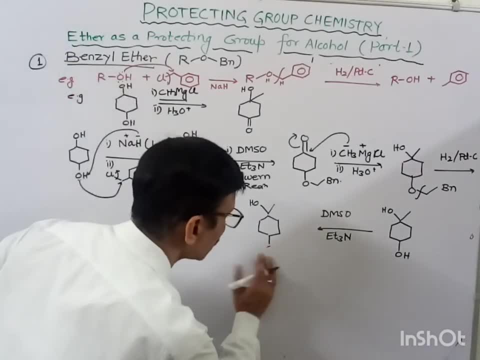 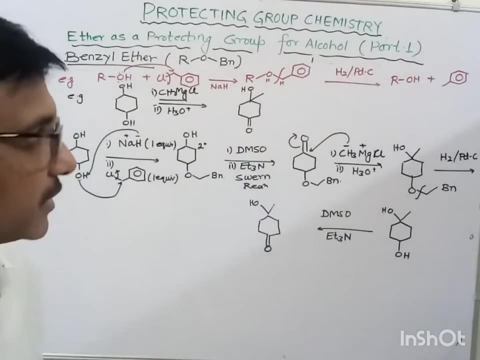 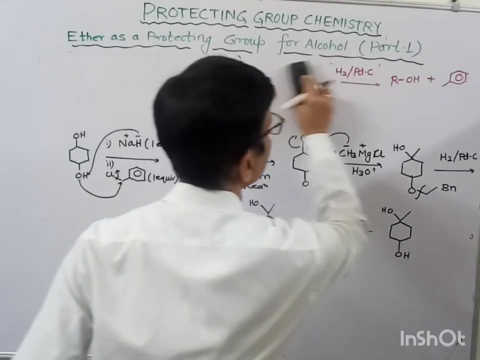 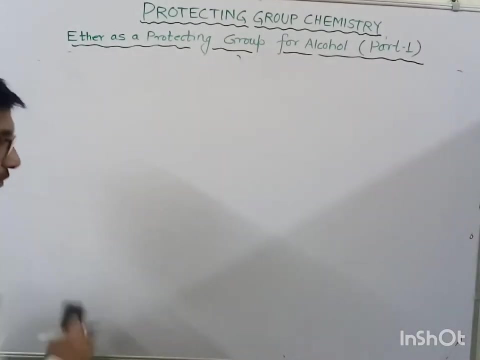 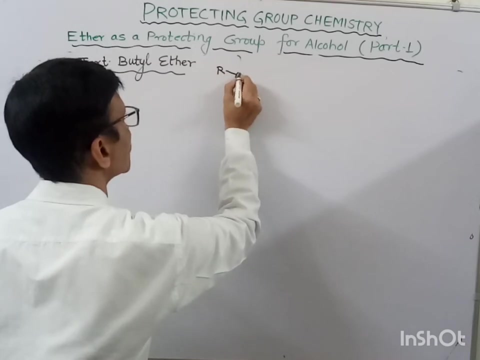 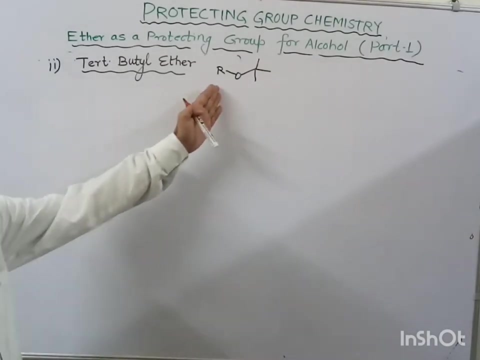 you. it may end up oxidation to give, so sorry, so oxidation to give you. so this is the example for benzyl ether. now let's come to the another protecting group. that is firstly, good I either, does she go down? so for this, the reagent, use this, yeah, I have told you I should be telling. and the acidic. 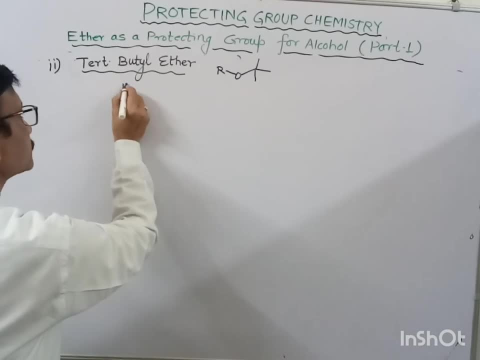 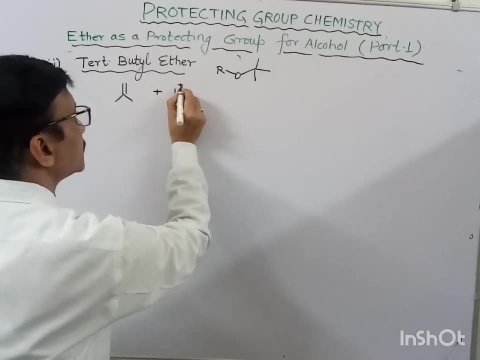 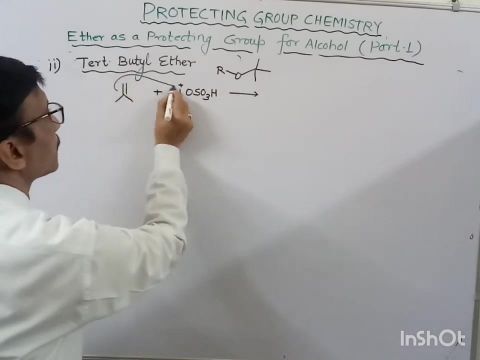 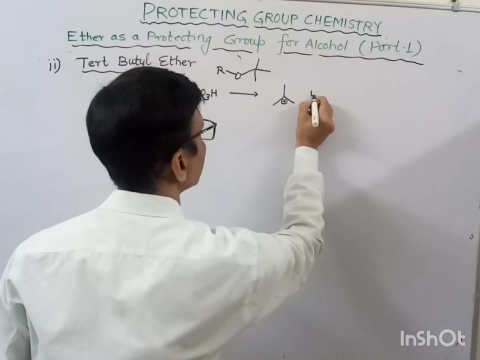 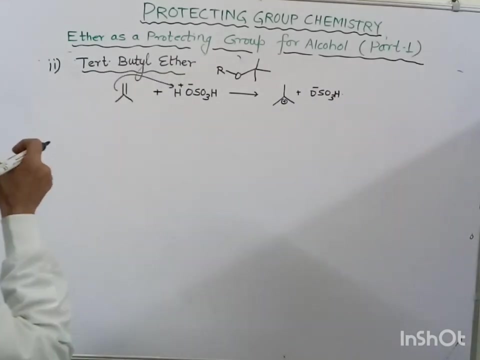 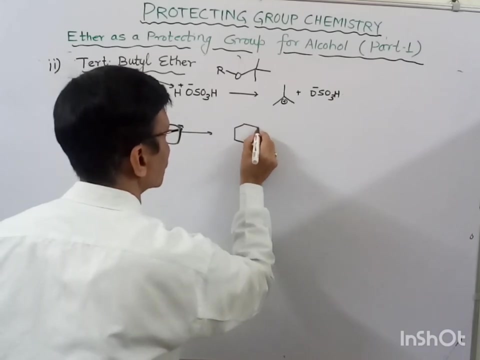 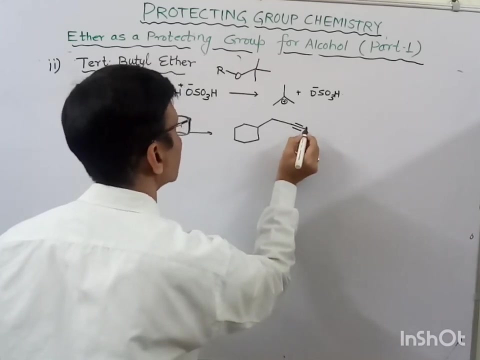 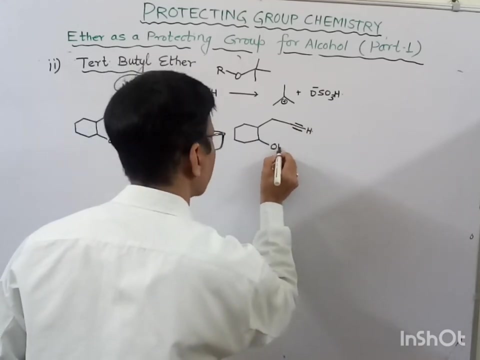 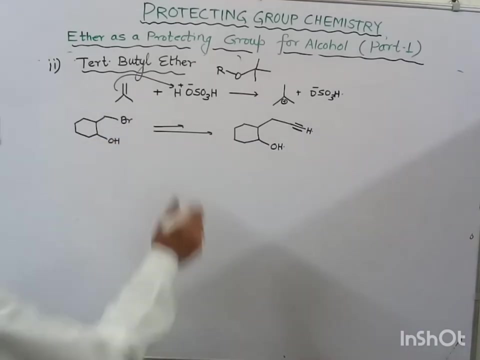 condition that can be used, suppose if we have isodutylene in presence of a stress of four. now, if we have supposed any ROH group, suppose I am taking one of the example- and if we want to convert, okay, suppose if you want to add, well as it like group, and if this may be added, we know. 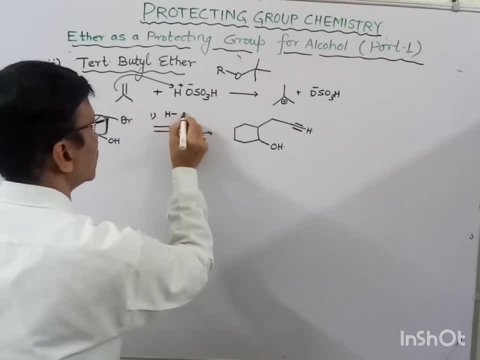 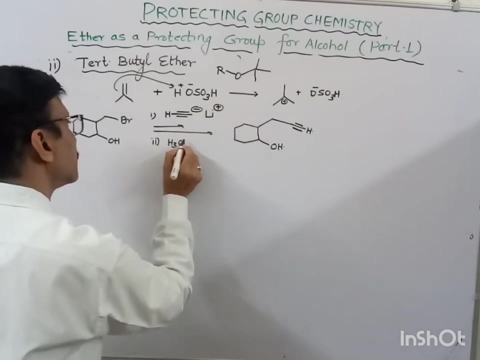 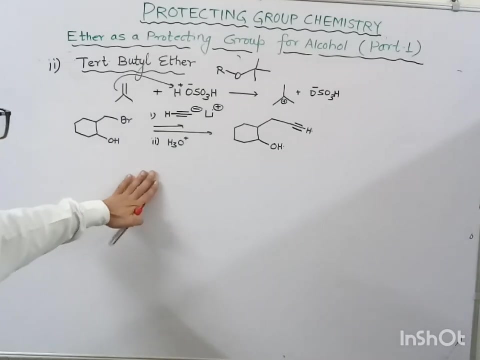 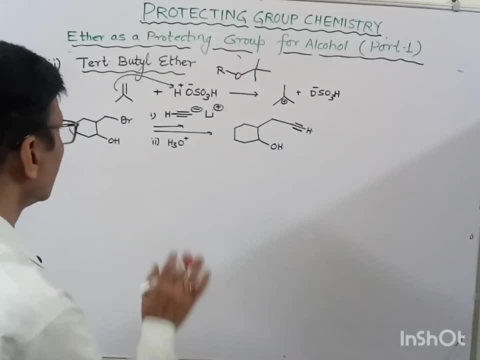 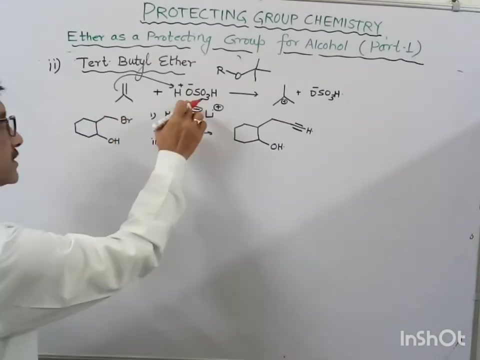 we can convert this into this. So, as we know, if this is reacted with this, then here this acetylide, it may act as a nucleophile also and if we act as a nucleophile, this will attack over here and this bromine that will be leave out. 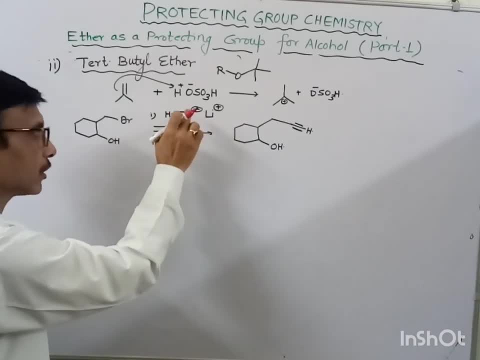 And this can also act as a base. This can also act as a base and it will extract this acidic hydrogen. So, no doubt, first of all, it will extract this acidic hydrogen as this acid based reaction being produced Faster. So this will first remove this acidic hydrogen and then the reaction will go on over here. 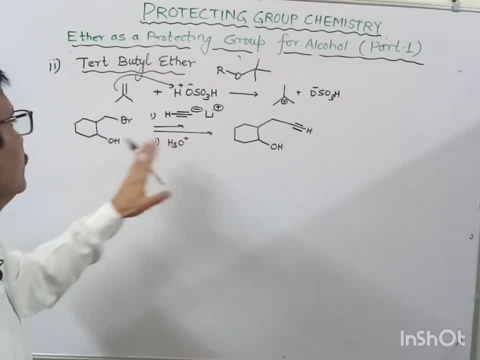 So we will not get the desired product. So, first of all, we should protect this OH probe, and we may protect it with the help of, we may convert into the Tulski butyl ether. So let's see the conversion. Let's see the conversion. 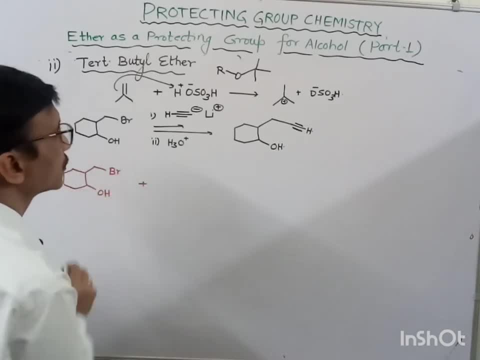 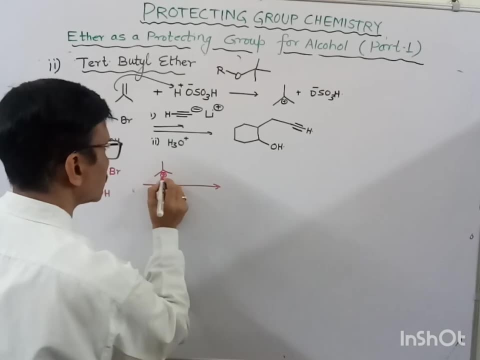 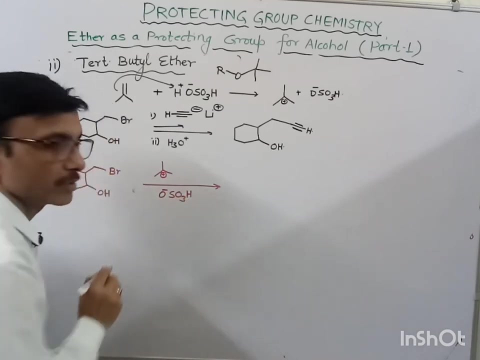 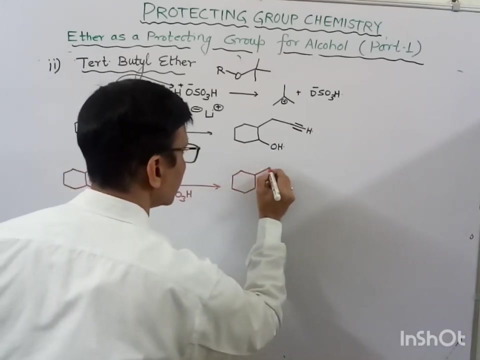 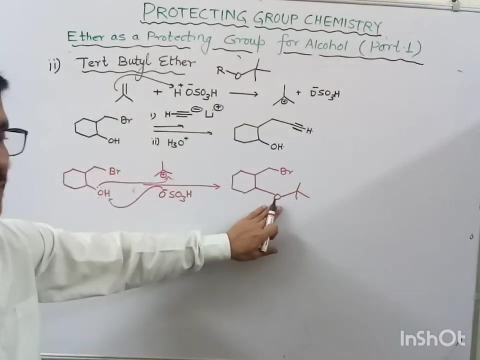 So we have, So this may act as a base and it can remove this acidic hydrogen and this will attack over here And we make that bromine over here and we will get here the Tulski butyl ether. So this is converted into Tulski butyl ether. 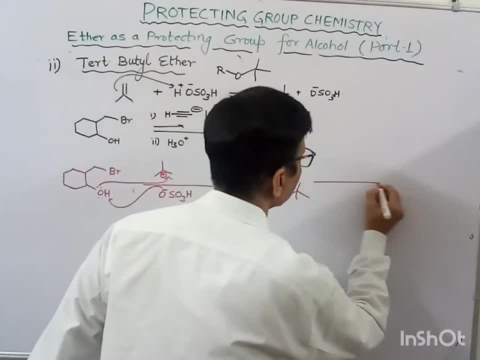 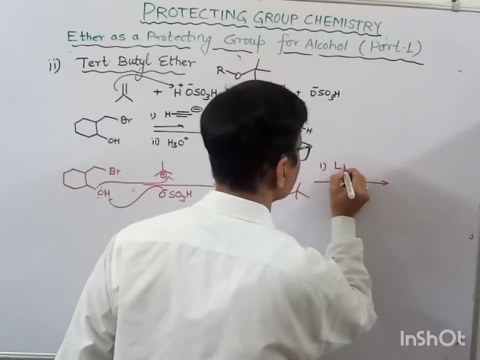 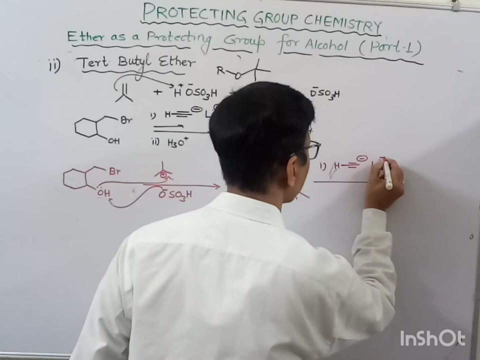 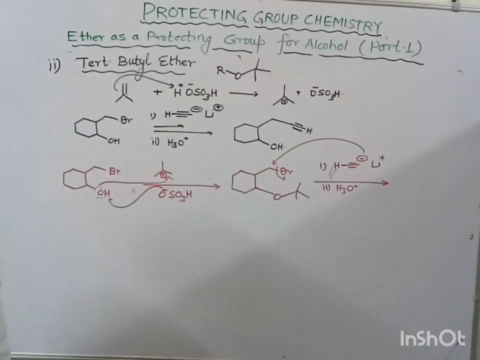 This OH is converted into Tulski butyl ether. now we can. we can react it with lithium acetylide, See So�. So this is how it then kicks on to the main brawling unit for some cooking. OK, So finally what we will get. 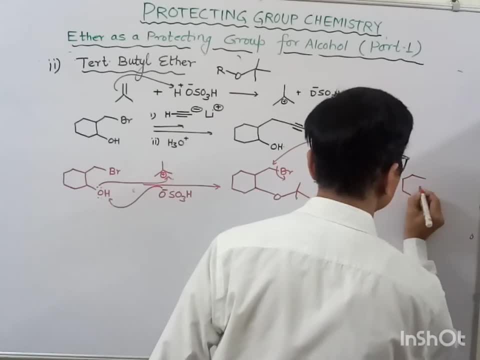 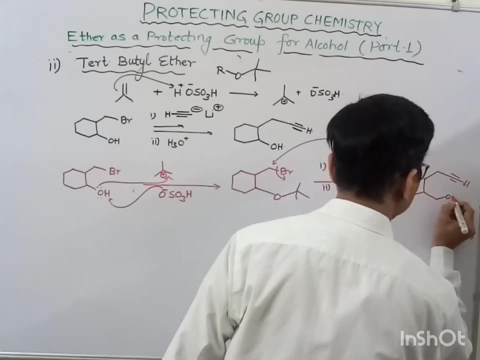 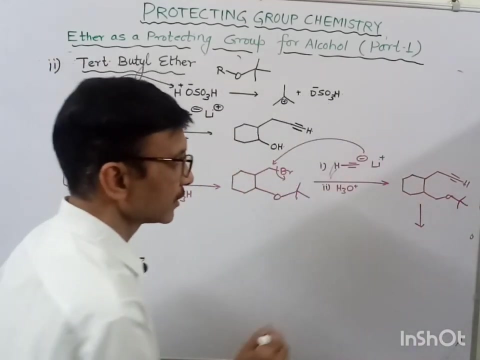 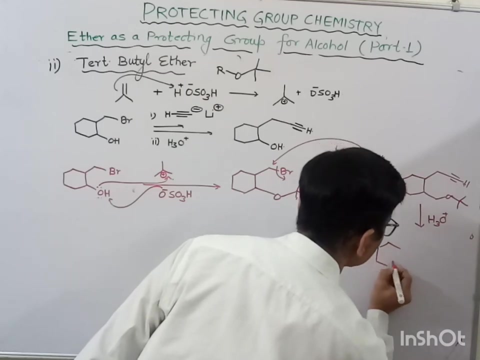 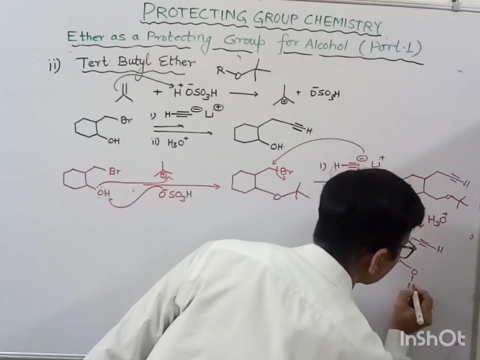 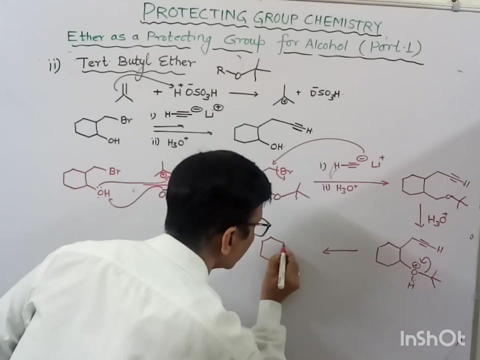 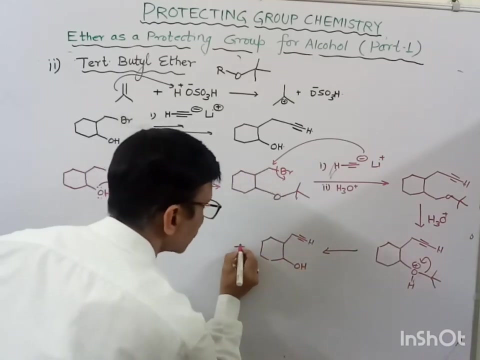 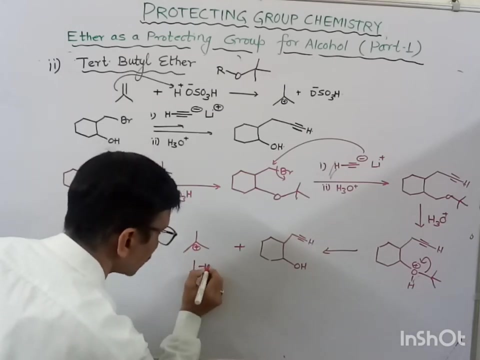 So this is basically our water now we can be protected. we can be protected under acidic condition. it may be deprotected. so this will this tertiary butyl group that we leave out, and we will get our desired product, one of the H plus that may be removed, and we will. 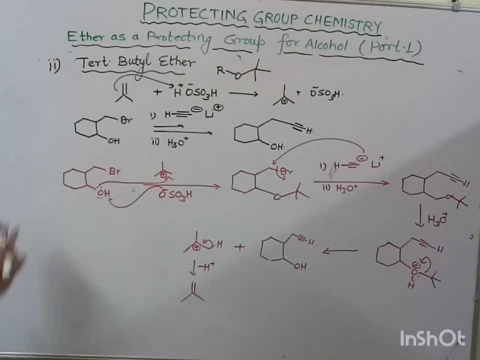 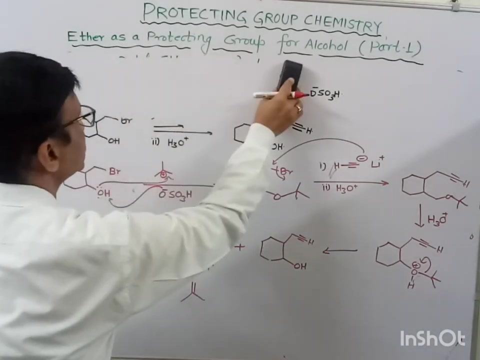 get our desired product. one of the H plus that may be removed and we will get our desired product. so this is one of the example where the tertiary butyl ether, the alcohol that can be protected by converting it into the tertiary butyl ether. okay, so let's see the third one, that is, PHP. 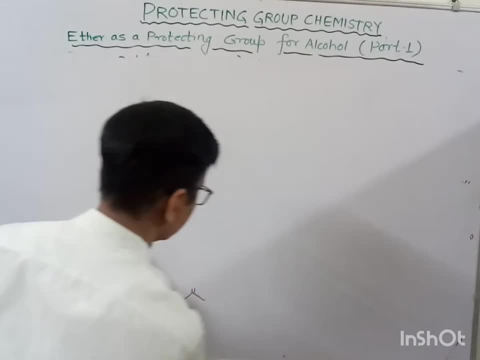 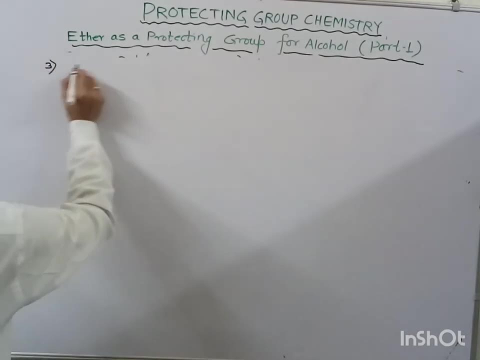 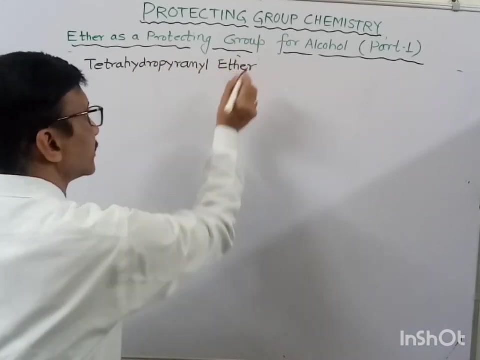 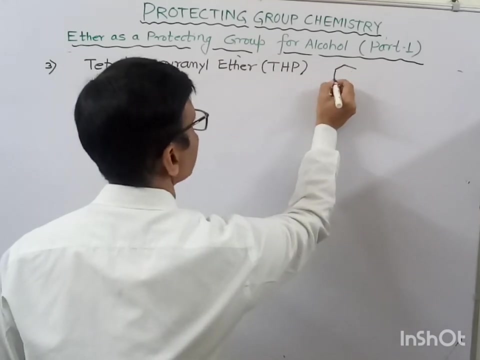 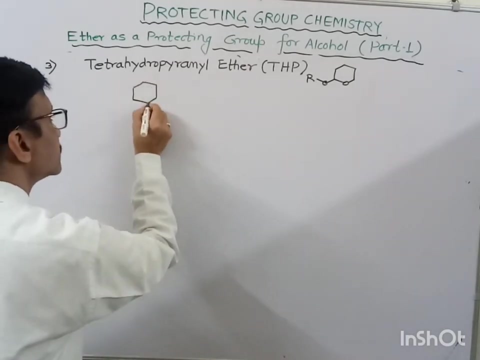 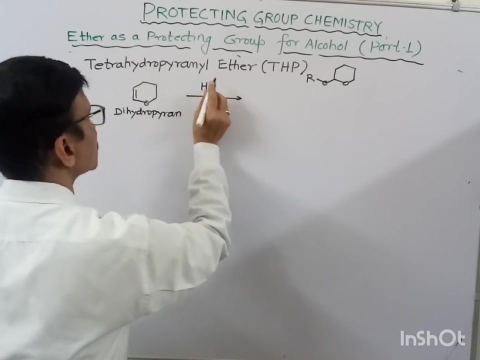 so this is one of the example where the tertiary butyl ether gets Our time. So, So, So, so, so, so so, and we may represent it by: so the reagent that we may use is dye. this is your dihydropyrone- dihydropyrone or in acidic condition and this anhydrous. 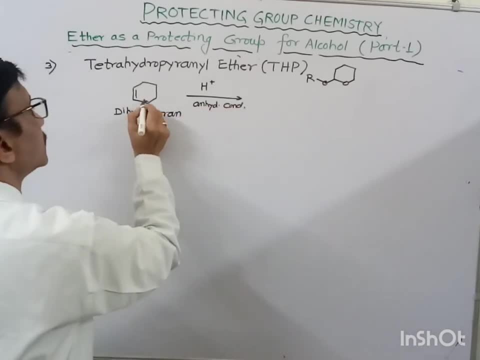 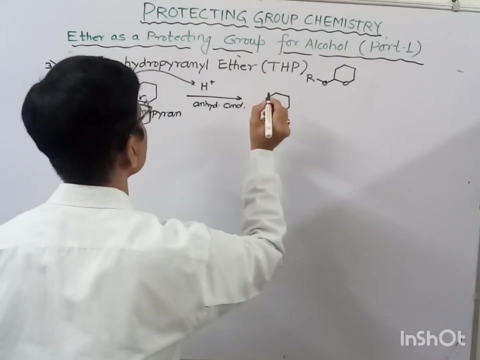 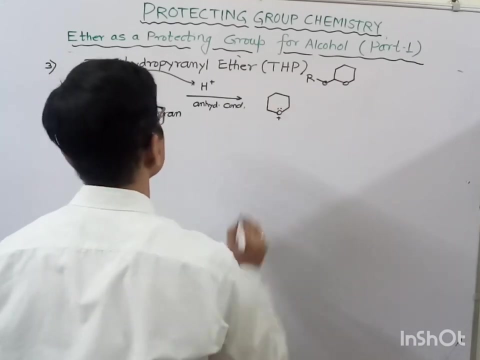 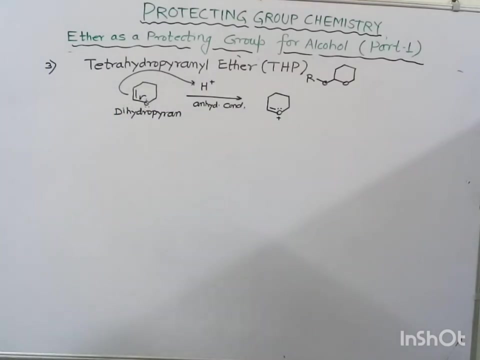 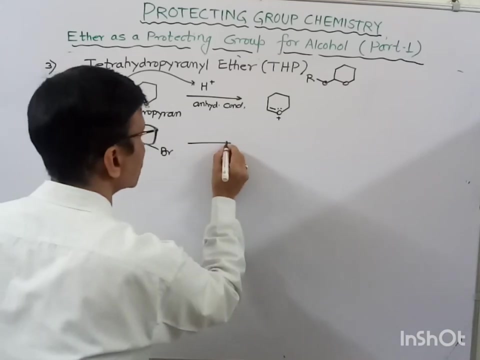 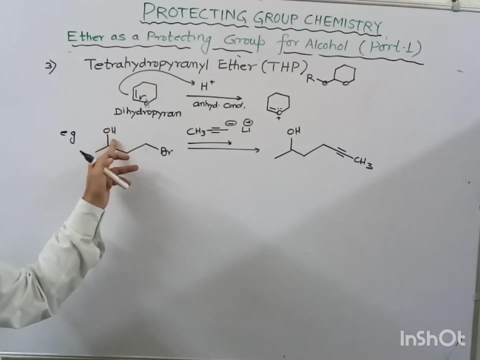 condition here. okay, so what we can write? okay, now suppose we have, now suppose we have any alcohol. now suppose, if let's take the one of the example, let's see one of the conversion. so suppose this has to convert it into. so, first of all, this will act as a base and it can extract the acidic hydrogen. 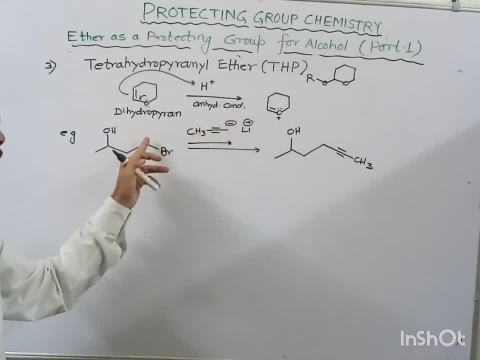 and then there is an IQ value of the dry oxygen water 기록장, which here is affair곡. So first of all this will act as a base and it can extract the acidic hydrogen, and then it will it may act as a nickel file to add substitute over here via this SN2. 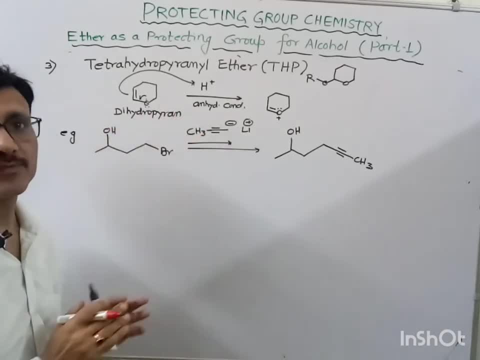 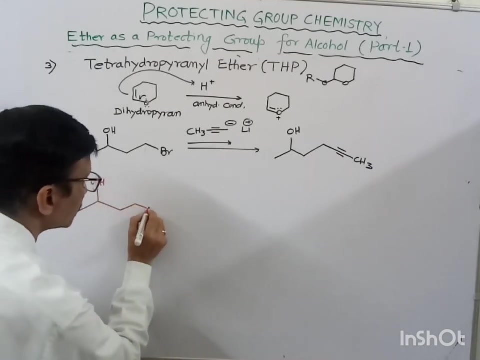 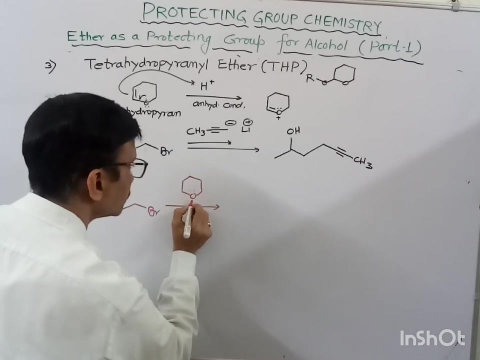 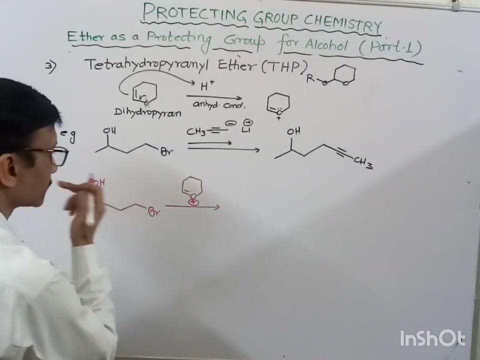 reaction. so, first of all, as this SN2 reaction being fast, as I told you, so this should be, this OH should be protected. so let's see first the protection using this THP, so let's see the mechanism. so we have. okay, so now. okay, so now. 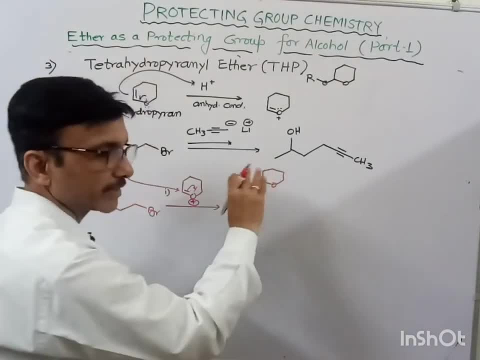 okay, so either here we can write a THP only, we can write a THP only here. in case of this we may write the THP also. so okay, so now, either here we can write a THP only, we can write a THP only here in. 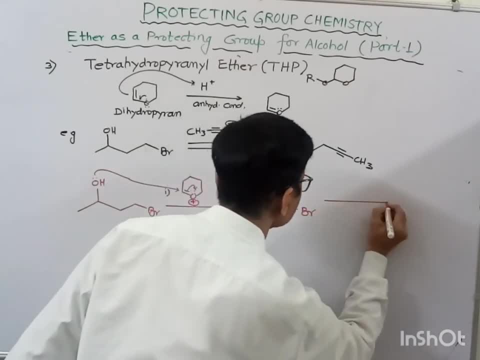 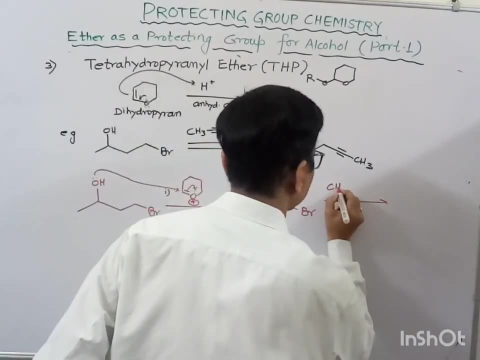 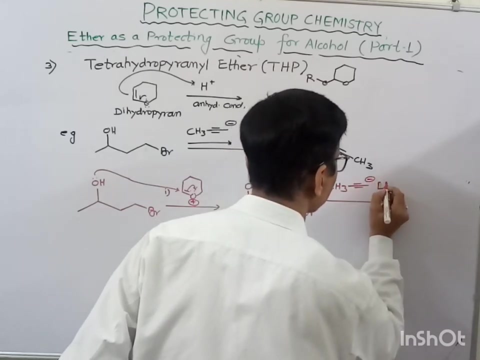 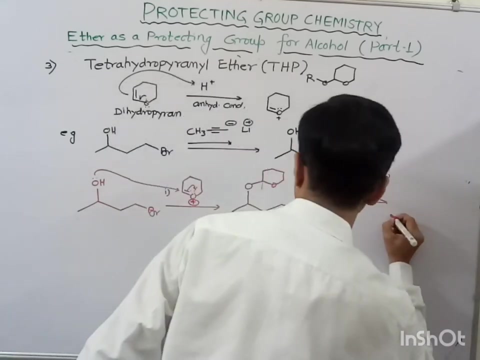 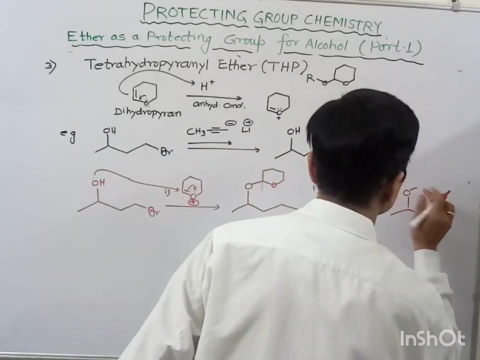 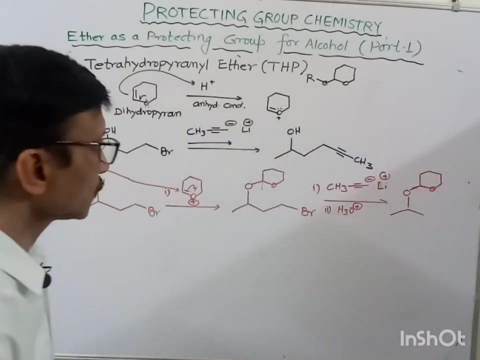 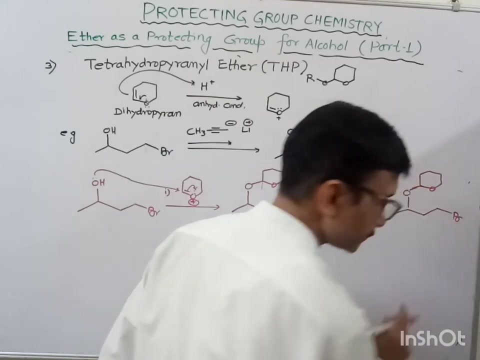 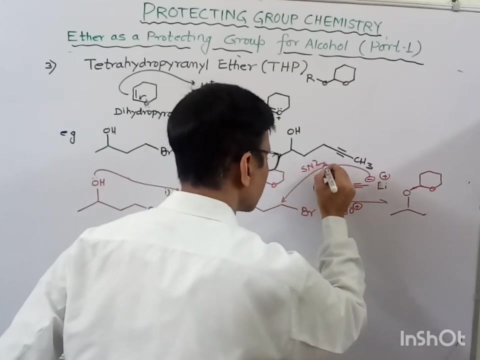 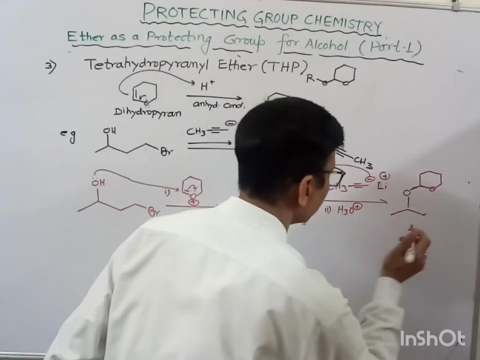 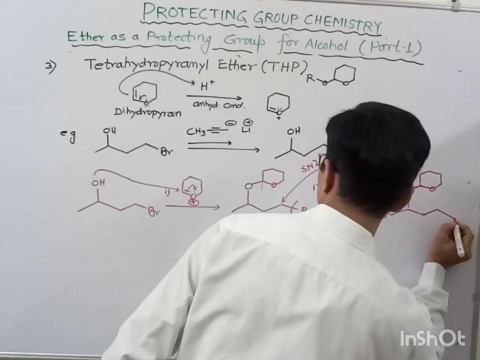 so here I have protected this OH group. now this can be reacted, okay. so here I said, by this ascent to reaction, this will attack at the back side and we have this is this to be in believe vote and we will get the nucleophile will add over here, okay, and in next. 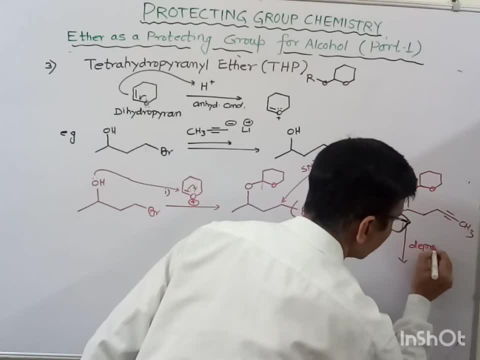 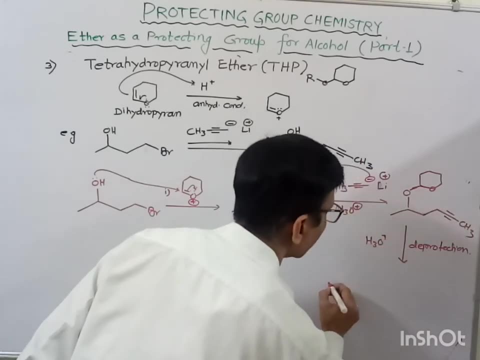 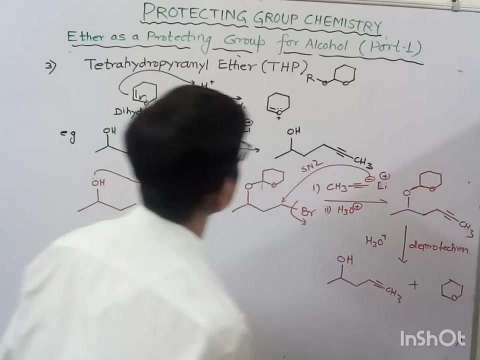 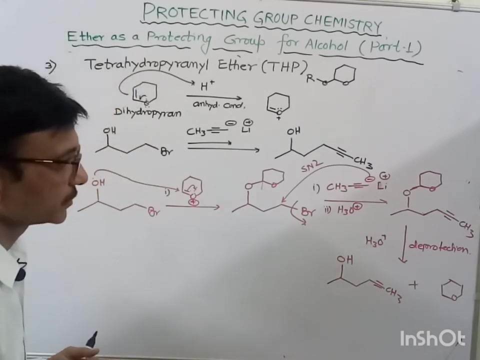 step. we can be protected, so the production can be done using acidic condition. we can be protected and you, you, you, okay, so like this, so it may be be protected in this way now. so this is about the PHP, PHP as a protecting to fall and call. now let's see the next. 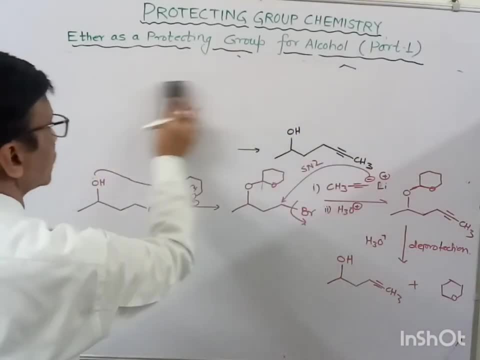 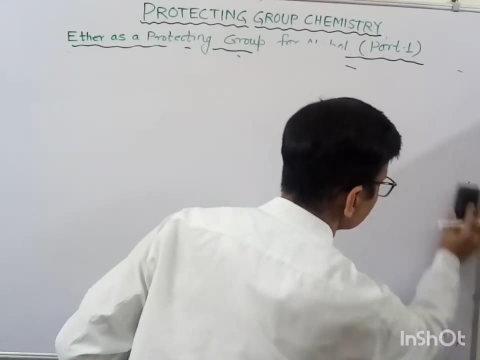 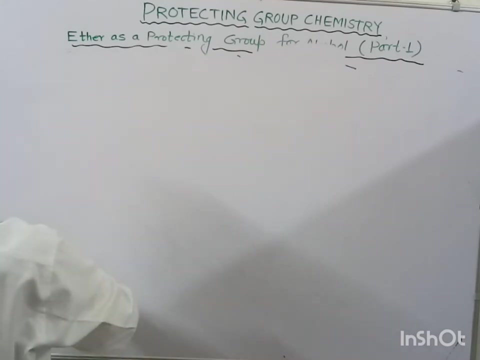 protecting group is the OH group. so this is the OH group, so this is the OH group. and is right, Mutile or tri alkyl sil corn trialtase o, three, three, C. we've got, we've got here all of that. high Depth is C, A, E. job, nobee. no like Oh km either the claro Sonica, so will. this would be retracted. this is tight and that is trial to have a full deja vu in seller's care on this text. it's available in the other, Sigrid in Palmy road, so this will have a full effect of it for several days. okay, this is trial to select� 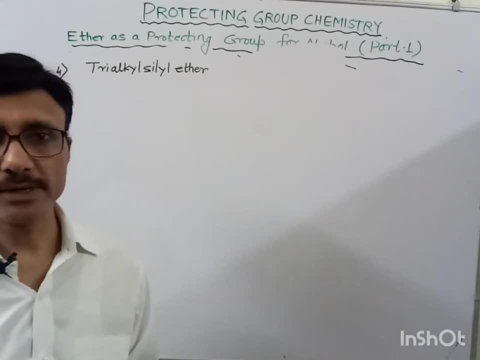 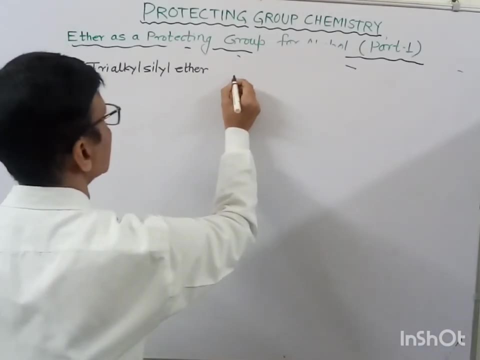 So I told you various trialkyl silyl ether. it may be TMS, TES and so on, I told you. So let us take the example of this. suppose if we have trialkyl trimethyl silyl ether. 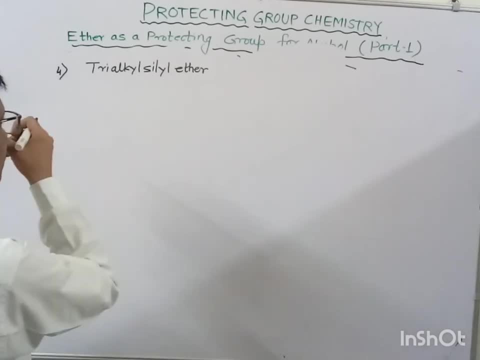 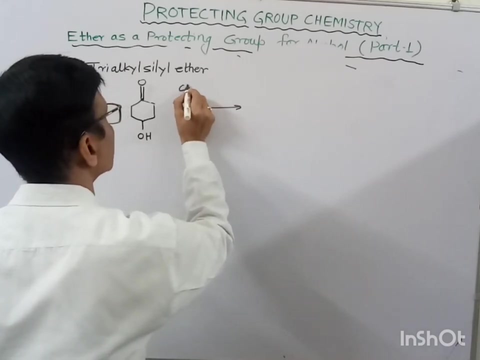 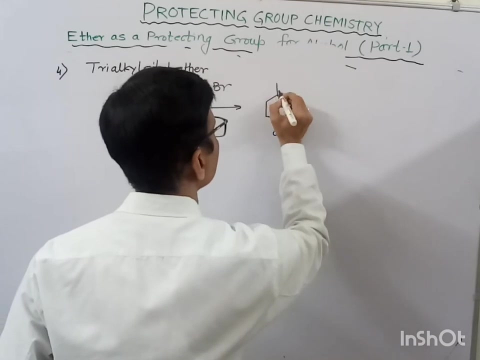 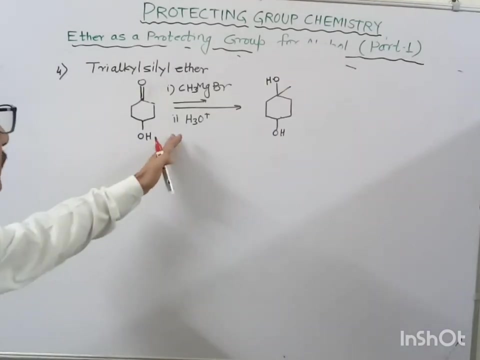 suppose, if we have trimethyl silyl ether and one of the examples that we may take for conversion, let us see one of the conversion that we may take, one of the conversion. Let us see one of the conversion. okay, suppose, let's see this conversion. so here, if we see, if we react with this, 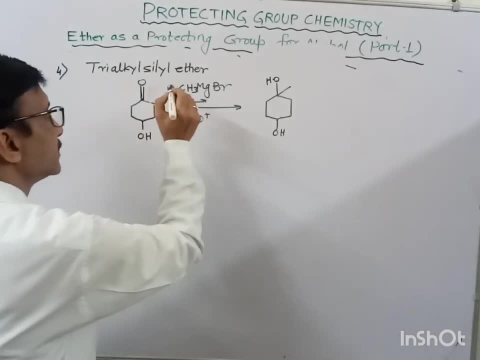 Grignard reagent. then what will happen here? this Grignard reagent, that will act as a nucleophile and it will act as a base also. so first of all this: it will compete. so this substrate will compete for this one and no doubt this H will be. 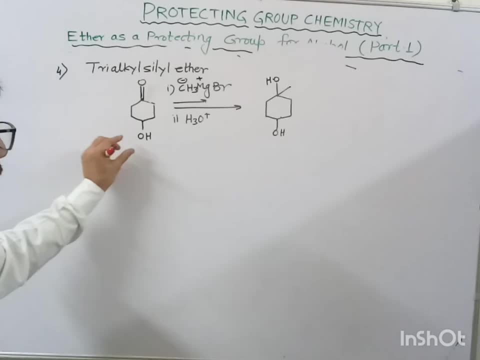 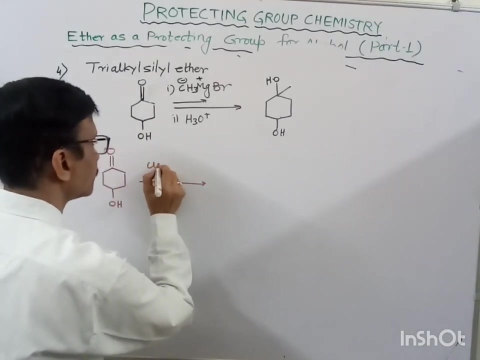 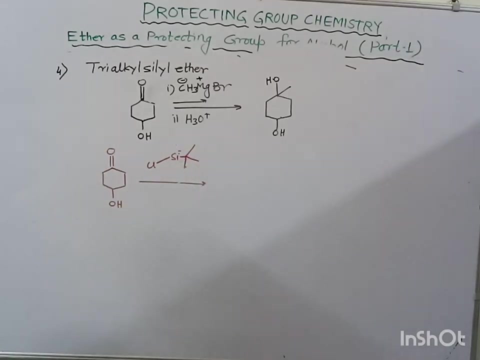 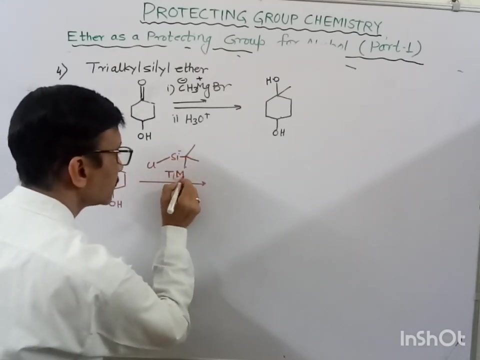 extracted first in comparison to this. so first of all, we should protect this alcohol group. so let's see the mechanism. so let's first protect it by using trialkylsilyl chloride. so if we have a trialkylsilyl chloride, okay, so we have a trimethylsilyl chloride. this is TES, trimethylsilyl chloride, and it. 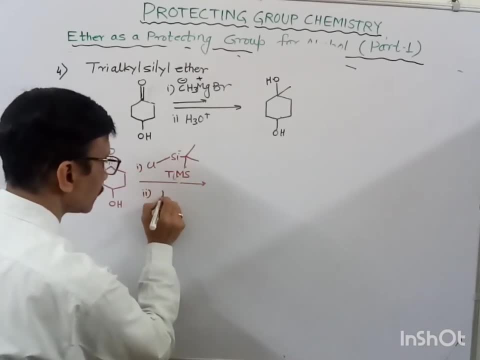 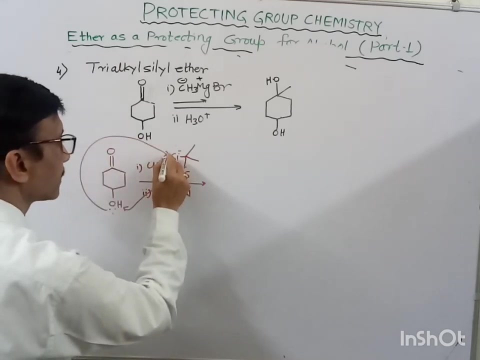 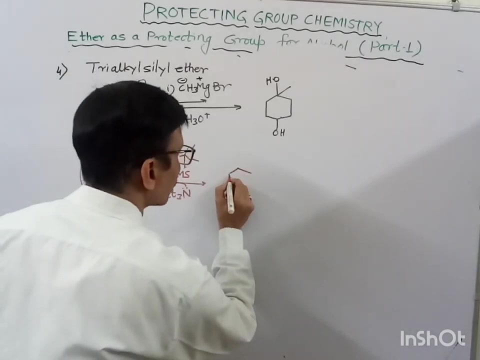 may be first of all using triethylamine. this OH group may be extracted out and then sucked throughout that pH and these NO2 NaOH group. for that reason right now there is a bond, let's say threeskih NH3 complicates with this OH group for 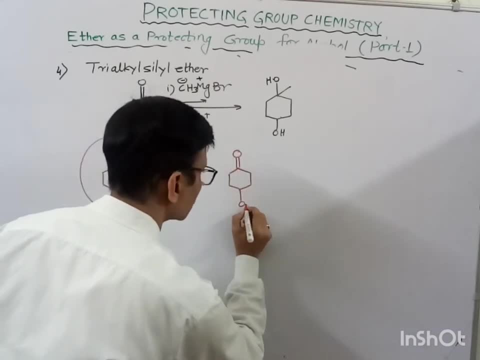 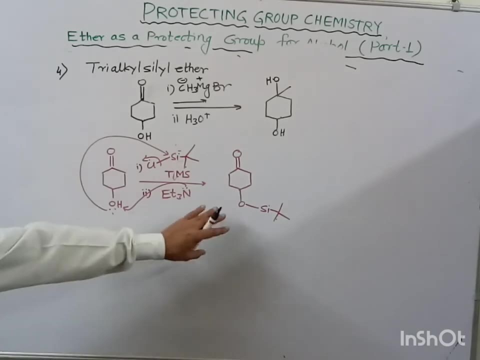 that. so it becomes� Armable- Ne இர음- Armable evaluativeения, armed with ADAM, who is used to rapidization of aидeneja reagent. Okay, so, So this is protected. now we have protected this OH group, and now it may be. 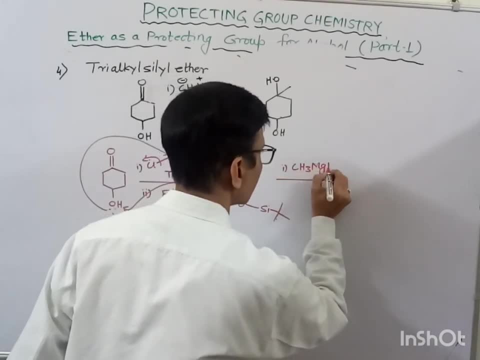 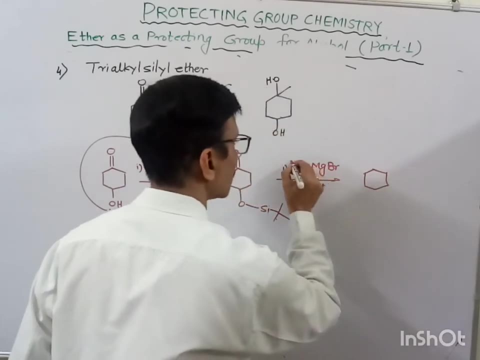 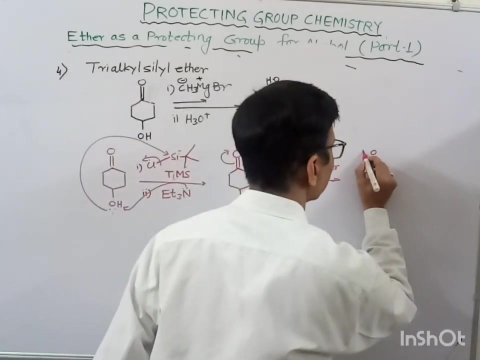 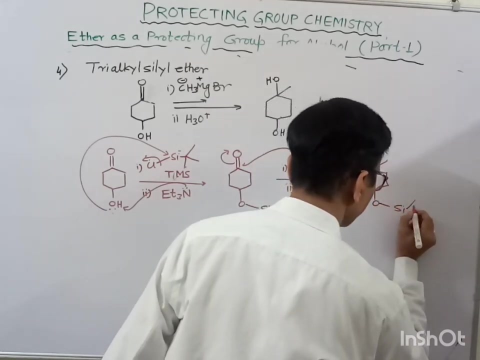 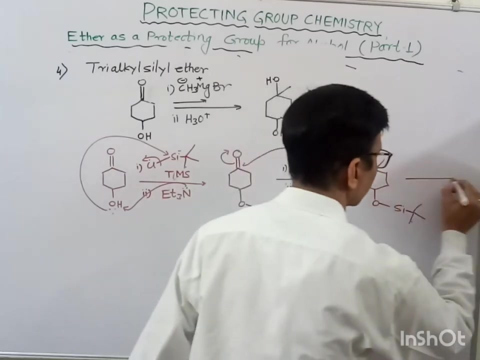 иковyeah with the Bernardi agent, followed by this hydrolysis. so here we will get OH and CH3 and now we have this tertiary butyl group. now we can deprotect it. so, as I told you, for this is silyl ether, trialkyl silyl ether, the deprotecting. 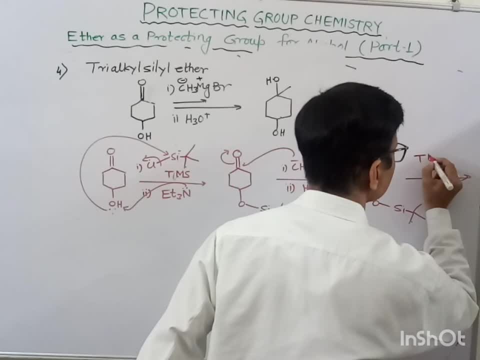 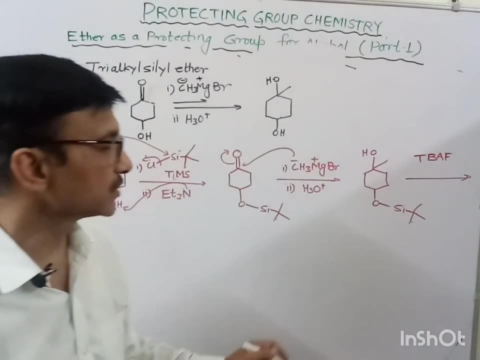 agent that we use is TBEF, so TBEF, this is the source of fluoride ion, so any anything which is act as a source of fluoride ion, so any anything which is act as a source of fluoride ion, so any anything which is act as a source of.